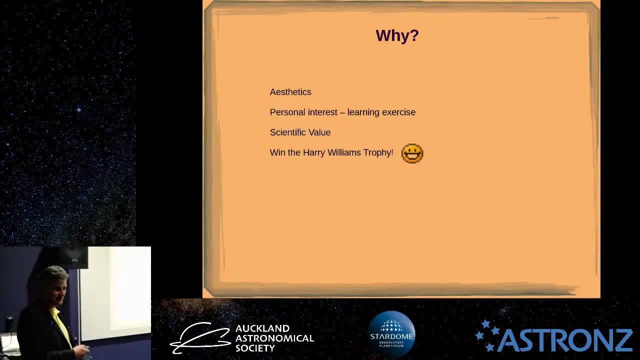 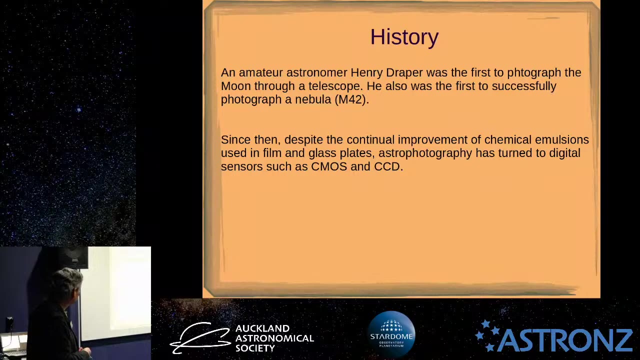 Right, yeah, It's way too bright for the telescopes. And, of course, you can have a chance to win the Harry Williams Trophy, the New Zealand Astrophotography Competition. Okay, Just a quick history. Henry Draper actually was, I believe, the first person to photograph the moon and also get a picture of the M42,. 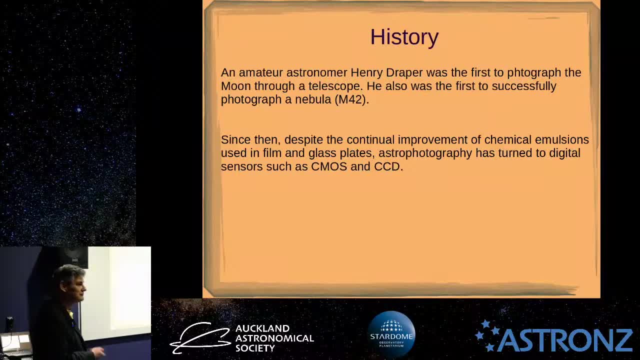 the great nebula in Orion, and that was of course using a very early version of film emulsion-type photography. But that's pretty much in the past now. I don't even know if you can buy that stuff anymore- probably specialist places. 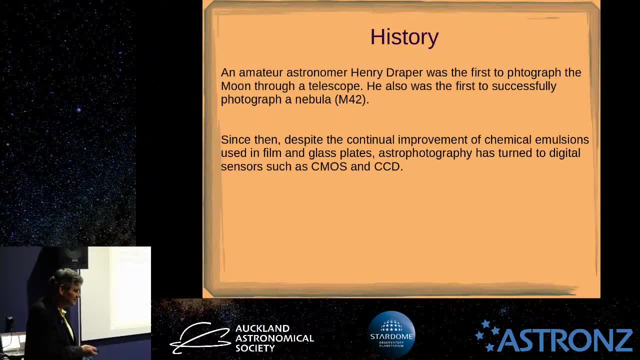 But everything has gone digital and there's two main sorts of digital sensor that are around. Pretty much all consumer cameras these days are using what is called CMOS, Which is the type of technology used in the sensor, and the other one is the CCD, which means charged coupled device. 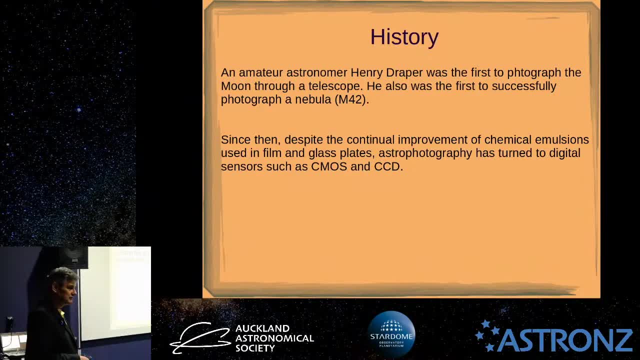 And that's mainly used for scientific work because you get a really linear readout which you may not get from the CMOS devices It stands for, I think it's complementary metal oxide semiconductor, and those are used for similar technology for computer memory. 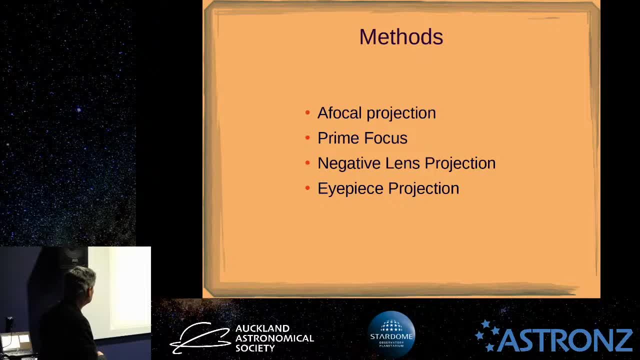 Chips and all sorts of things. Okay, so there's a few different methods you can do for astrophotography. We've got a focal projection, prime focus imaging, negative lens projection and eyepiece projection. So why would you do those and what are they for? 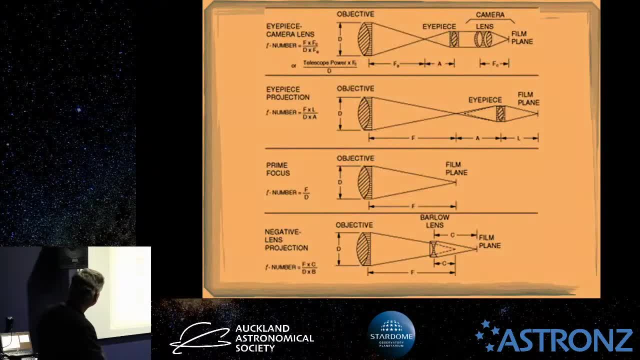 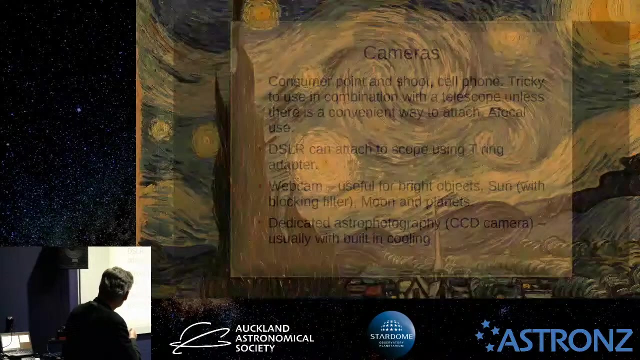 So we'll take a look at each of them. So this shows you the arrangement, The arrangement of your optics, with your camera stuck on the back. So, for example, here this one at the top- you can see where you've got a camera with a lens and an eye. whoops, I'm sorry. 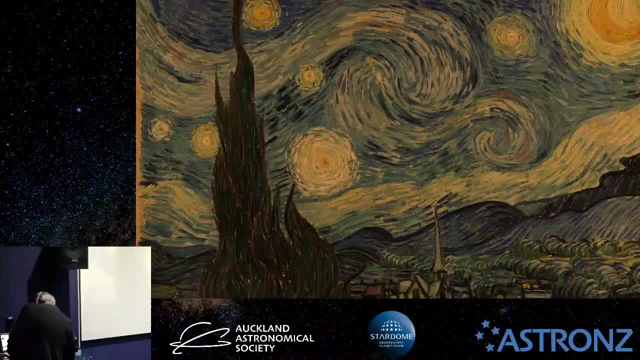 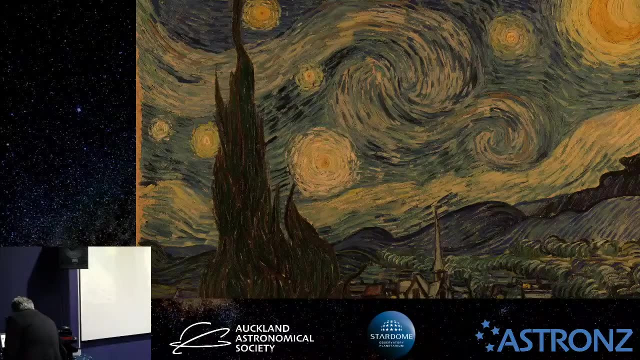 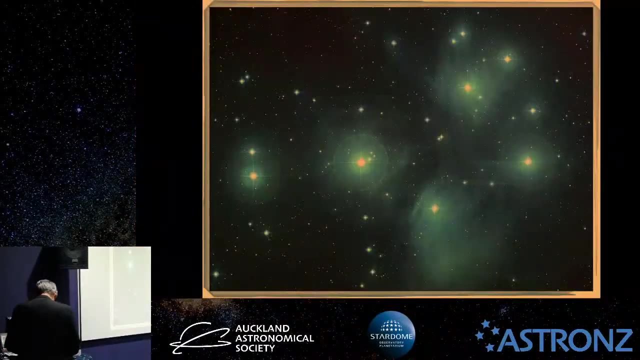 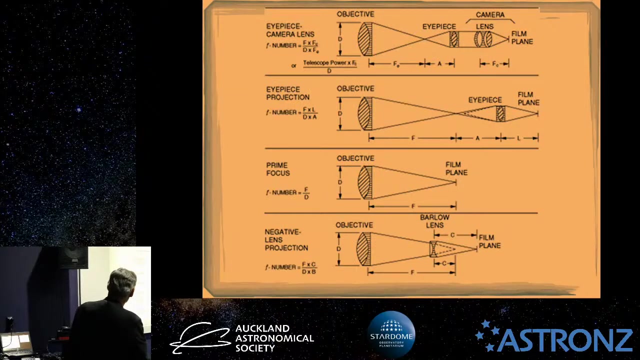 What have I done here? Sorry about that. It is Press the wrong button, Okay, it's off Control of the liquid. Okay, All right, sorry about that. I accidentally closed the thing down, so Okay. So you've got the afocal projection at the top, there where you have a lens, telescope eyepiece and objective. 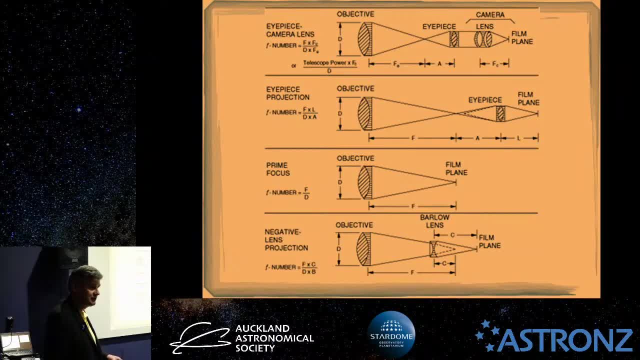 And the example, And the example where you'd use this is with a smartphone camera. it's obviously got a lens in the camera. you hold it up to an eyepiece and so that's a really simple way. people find that they can get quite reasonable images of the moon doing that or anything that's bright. 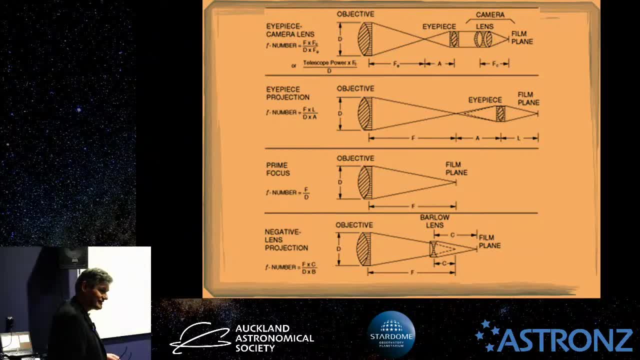 I wouldn't attempt it for faint objects. it would be probably wasting your time unless you've got a really good way to control the focus and long exposures and so on. And then there's eyepiece projection, which you see. there you basically have the objective lens and eyepiece still, but a camera without a lens. so I don't know, has anyone tried that method of imaging? 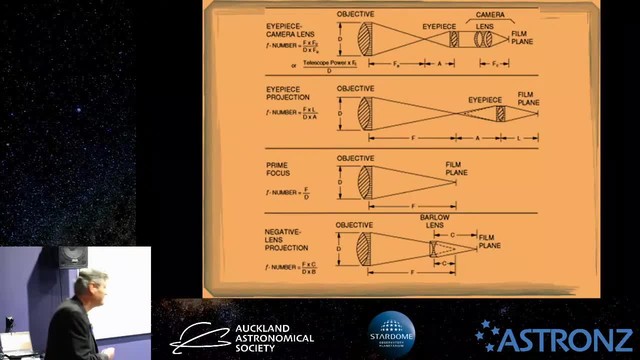 Probably you have Sean. Okay, how did it go? Just one mistake? No, Okay, So then the most, probably the most common one is prime focus. Okay, So then the most, probably the most common one is prime focus. 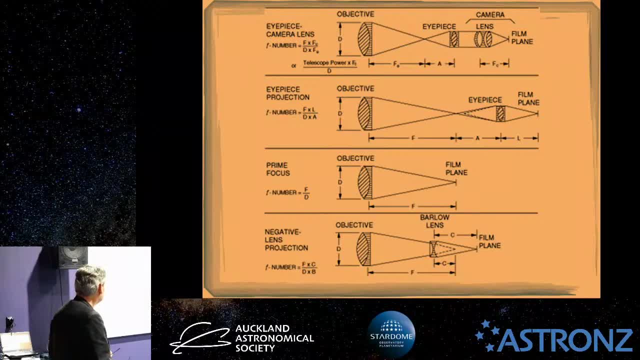 Okay, So then the most, probably the most common one is prime focus And there's a lot of prism imaging, where you have your objective and which is basically a telescope with a camera attached to the back with no other optics. maybe a corrector, perhaps. 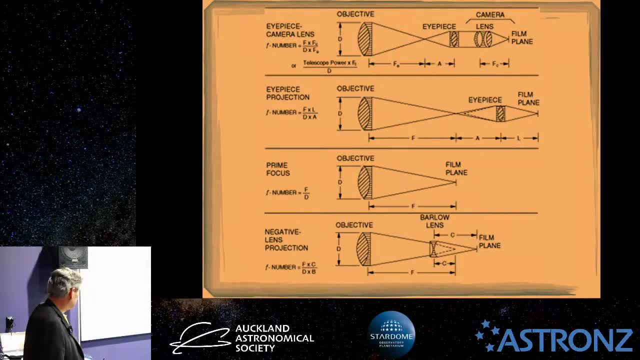 So yeah, that's probably the way most people do it, But you've got this one at the bottom called negative lens projection, And again you have your objective lens and you have a negative lens projection And you have a negative lens, which we mean a Barlow lens, effectively. 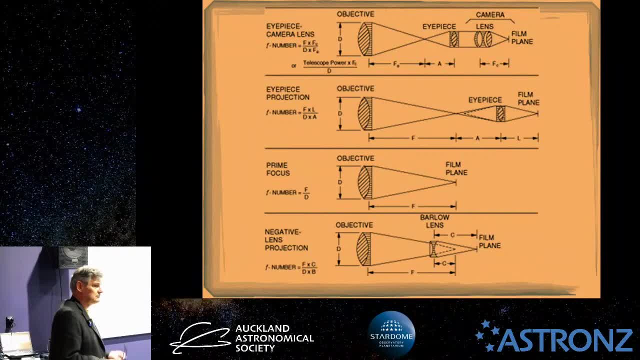 and then your camera, And this is quite common still, because what it's used for is if you're doing planetary imaging or imaging something really small- like a planet is quite small on the sky- and if you haven't got enough focal length in your telescope. 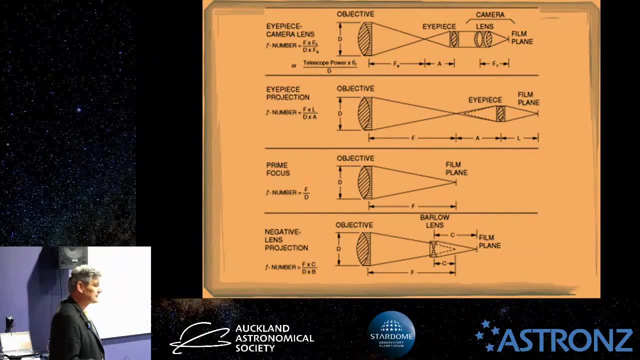 the image of the planet on your camera will be really tiny, So you use a negative lens to increase the image scale, and so that's pretty common with amateur telescopes. I'm pretty sure Sean does this all the time with his planetary imaging. 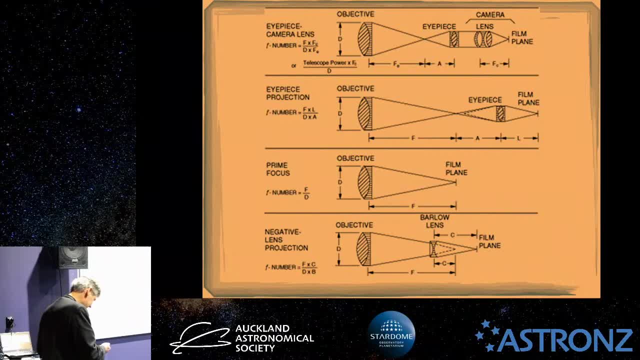 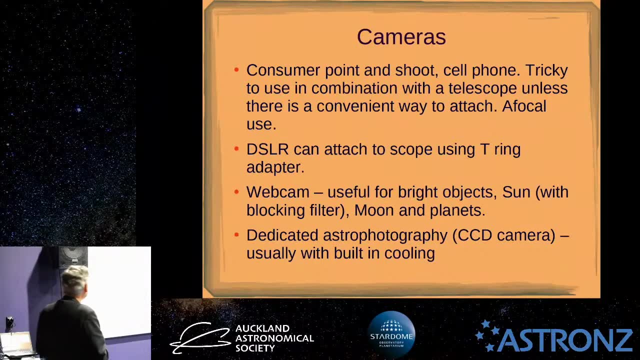 Barlow lens in combination with your telescope, Right. so you can use all sorts of different cameras: point-and-shoot phone, cell phone. They can work with bright objects, But if you're going to do anything a bit more serious, they're going to be difficult. 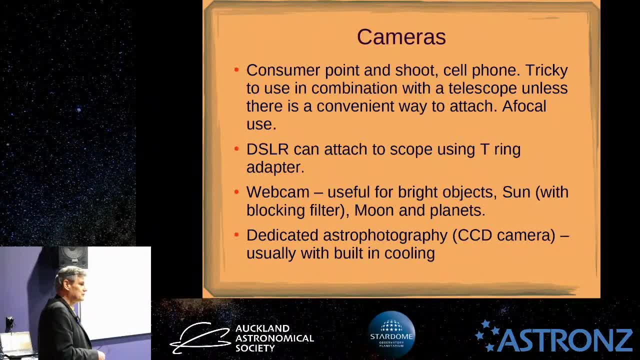 You can actually get holders now for cell phones, because one problem you'll have with a cell phone if you try to use it on your telescope is actually getting the camera positioned at the right place in the eyepiece to capture the image. But you can buy. I think Andrew is here. 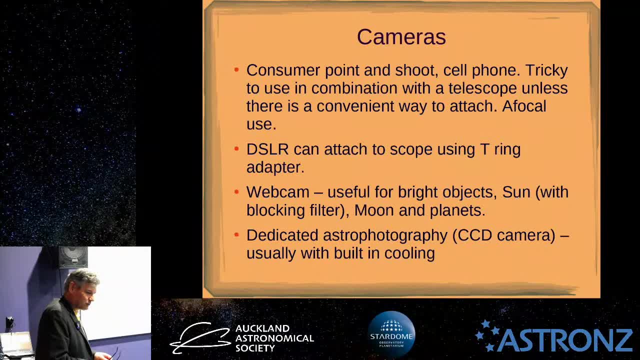 you guys sell these, don't you? Steve Holders for cell phones? Do you do any? If anyone's interested in that, see Andrew or Steve, Because a lot of people already have a phone. it's a good way to get started. 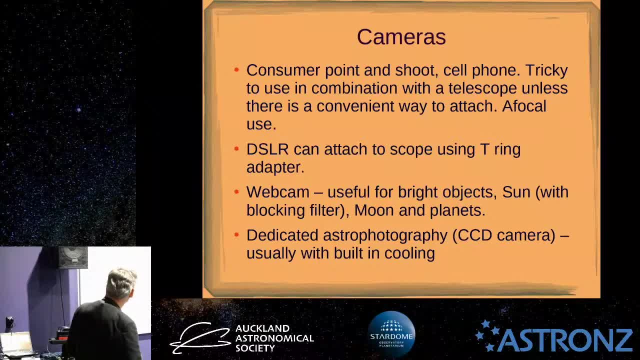 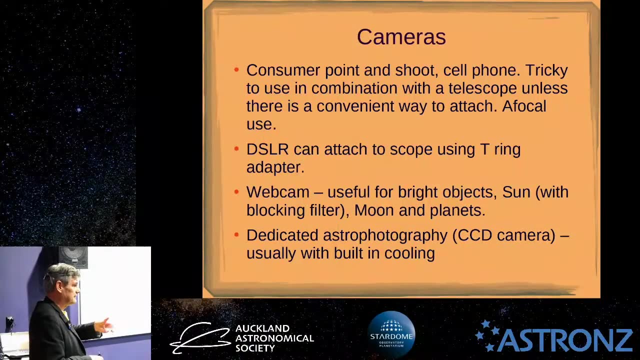 because you don't have to worry about buying a special camera. You can use a DSLR or actually one of the newer mirrorless cameras as well. The way they work is you need some kind of adapter because they have a connector for the specific. 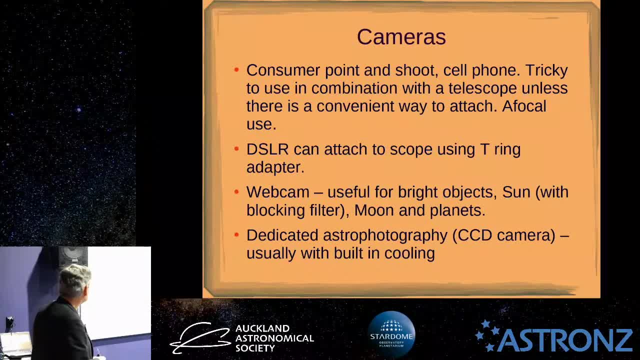 a camera lens for that brand. So, for example, Canon, Nikon, Sony, they all have their own connection mechanism for putting a lens on their cameras and they're not compatible. So you have to buy what's called a T-ring adapter and it's specific to your brand. 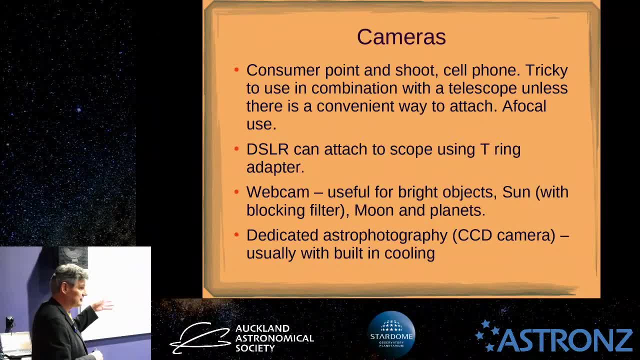 So if you've got a Canon camera, you have to buy a Canon T-ring and so on, and they're all pretty readily available, And again, Astron sell these Most brands fairly inexpensive. So what you then do? the T-ring then allows you to put an extension tube on. 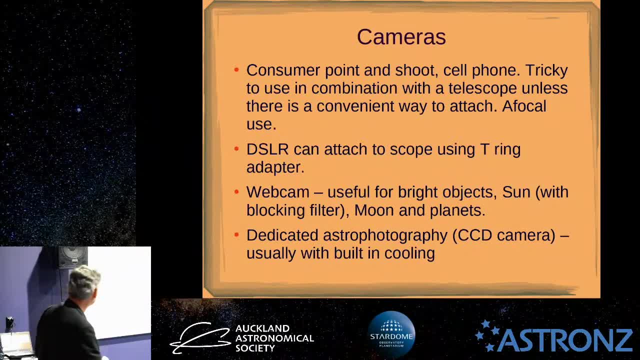 so you can fit it to your telescope focuser. Now, another type of camera that's basically webcams or specifically designed sort of webcam variants for this purpose is for imaging really bright stuff- sun, moon and planets. And the reason you use these 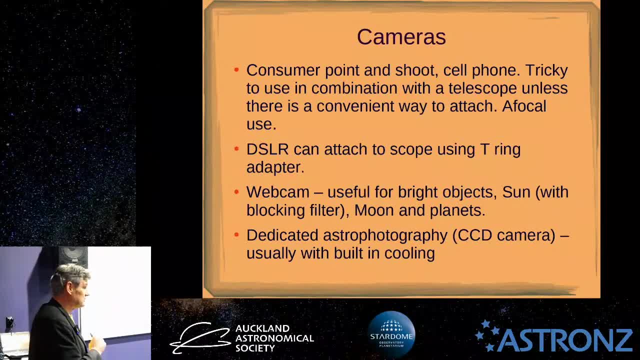 is that you're not generally capturing single images with these, but you're capturing movies. So you take an image of Jupiter or Mars and then you get a movie that you then feed into a stacking program. So it's basically a method called lucky imaging, because you pick out the good frames. 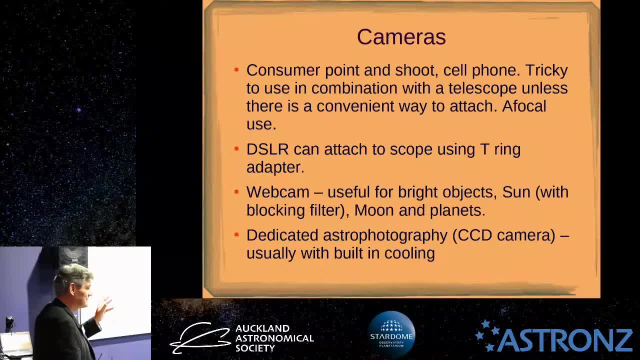 where the seeing is just stable for a tiny fraction of a second sometimes. so by taking lots and lots of images in a movie, you're bound to catch a lot of these moments of good seeing, and then you use software to stack them together, which we'll talk about. 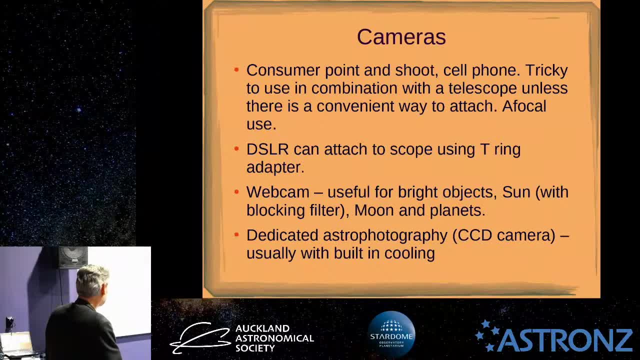 The other thing we've got here is a dedicated astrophotography camera, Often a CCD camera, but they can be CMOS as well. I actually brought one down. This one belongs to the Stardome And it's the CCD camera that's used. 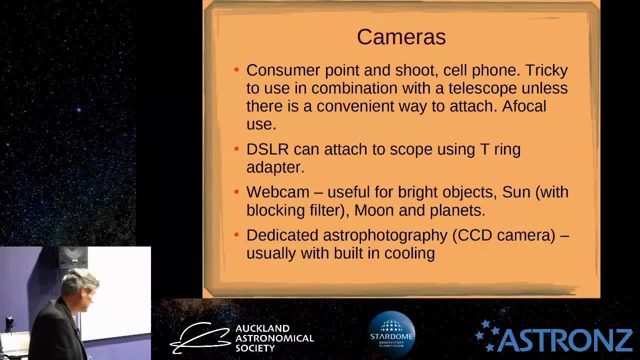 or can be used on the Zeiss telescope. It's not actually quite that big because the bottom part is actually the focuser, But that can fit onto the back of the Zeiss. But, as you see, they're a fairly large sized camera and they are expensive. 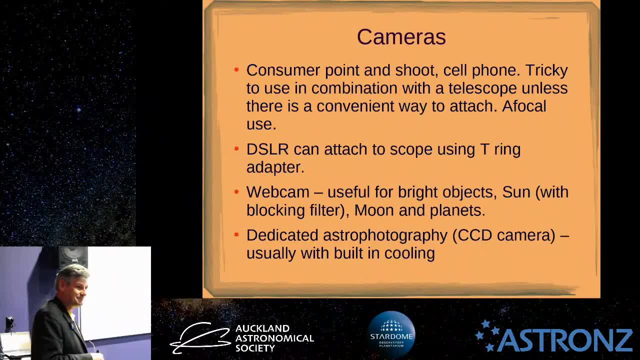 Do you know how much that one was Grant? I think the whole capital hurdle was probably about 15,000, 16,000 US. So yeah, Not probably a good starter kit But being a CCD camera, it's really designed for scientific purposes. 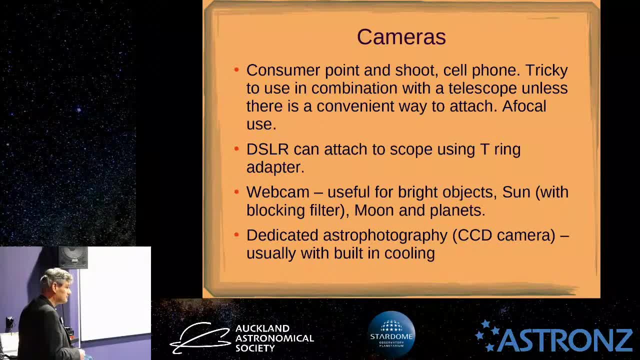 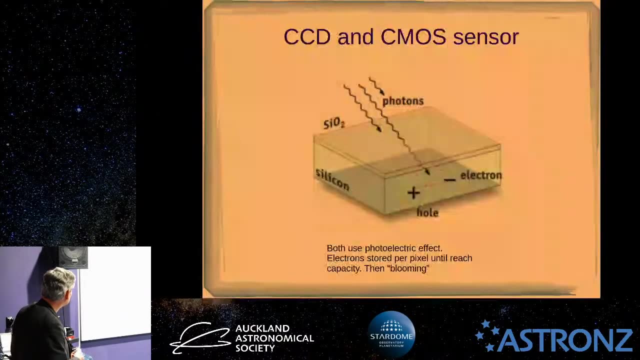 because you get really linear output and it's easy to calibrate the data coming out of the camera. So you can- if you're with Grant's micro-lensing team or doing other work, you can get accurate photometry OK. So this is a generic slide showing what these sensors do. 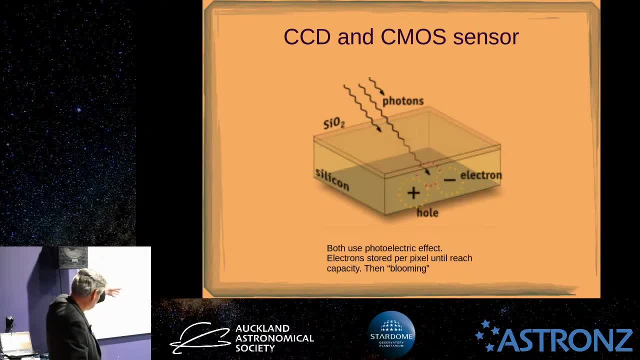 So effectively. photons come in, come into the little cell or pixel and basically the charge is built up until each cell has some capacity. and how much capacity it has will vary on the design: Usually a larger size one, if it's like a three micrometer one. 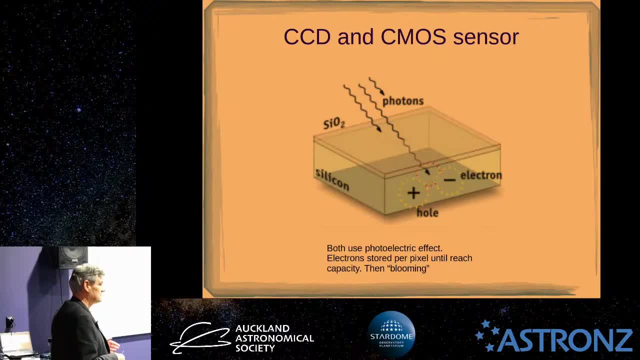 will vary on the design. It will generally have lesser capacity than one that's bigger at nine microns. So what that means is that a bigger pixel size you've got more dynamic range, So the difference between the faintest and the brightest data you can record. 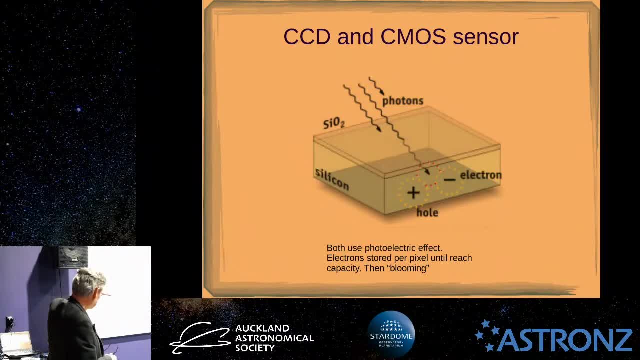 Once the thing fills up, there's a few things that can happen. Some of them have an anti-blooming circuitry that stops the thing doing anything at that point, But some of them will start bleeding into the neighboring cell. So the problem is the anti-blooming device. 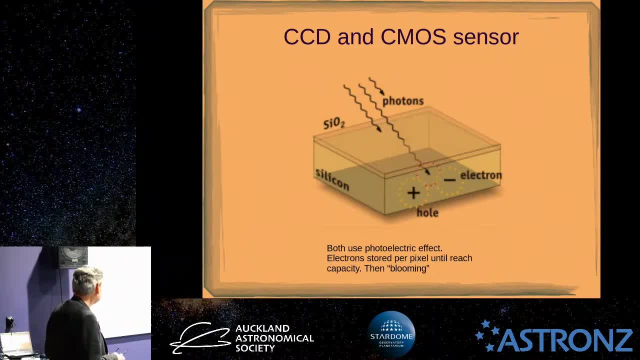 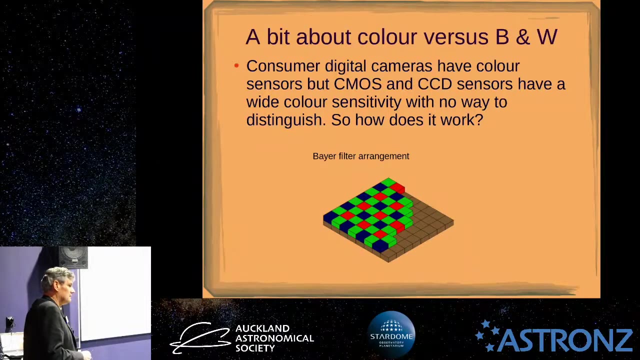 removes some of the linearity, So not so great for a scientific but probably for pretty picture stuff. So both the CMOS and CCD sensors actually sensitive to a range of colors, So they don't see red, blue or green, They just see a whole, all of the visual spectrum. 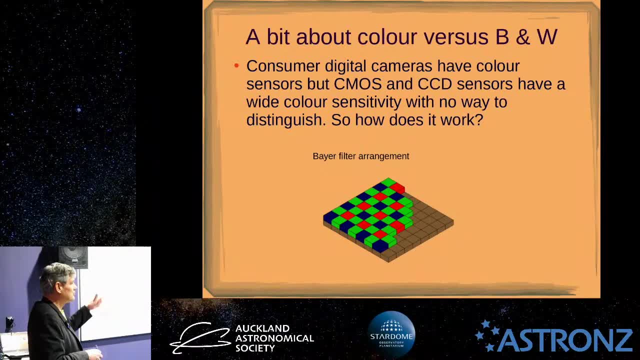 and a bit on either side as well, usually, But they're designed so that the peak sensitivity is usually roughly around the green, And the way if you buy a camera, you expect it to be in color. The way it works is that the array of pixels. 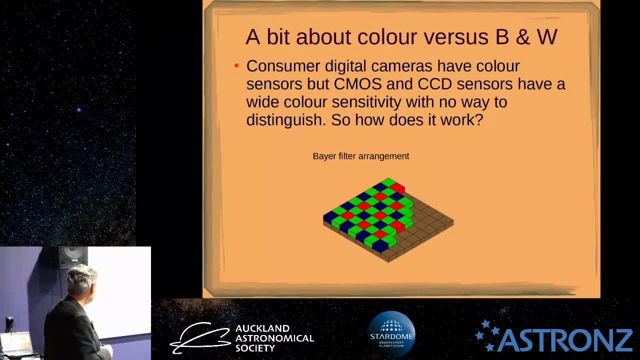 each has its own tiny little filter, So you have an array of red, green and blue filters. It's called a Bayer filter. as the usual arrangement, Each camera manufacturer will have their own secret formula for this, in terms of the actual filters that are used, 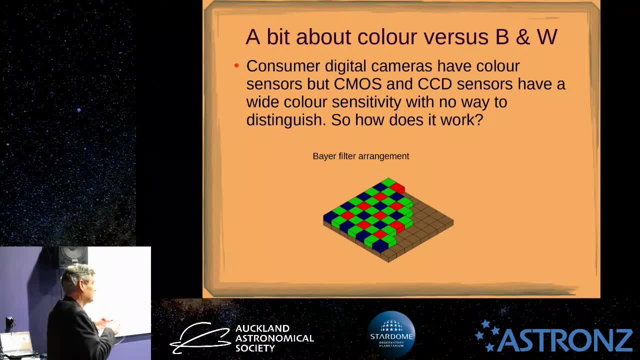 The particular where they fit in the red, green and blue part of the spectrum, and so on, And generally, consumer cameras also have as well as these color filters. they have what's called an infrared cut filter that blocks out infrared light. 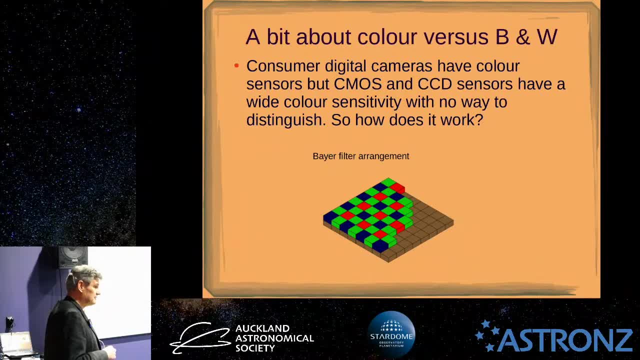 And this isn't a great thing for astrophotography because that tends to cut off some of the red And it's right where. I don't know if you know it, but the frequency of hydrogen alpha is down the red end, So a lot of nebula has hydrogen alpha colors in it. 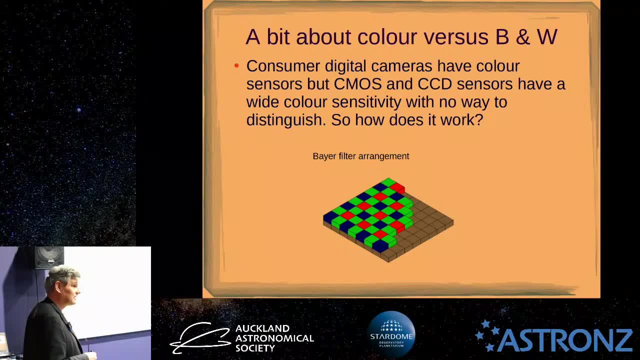 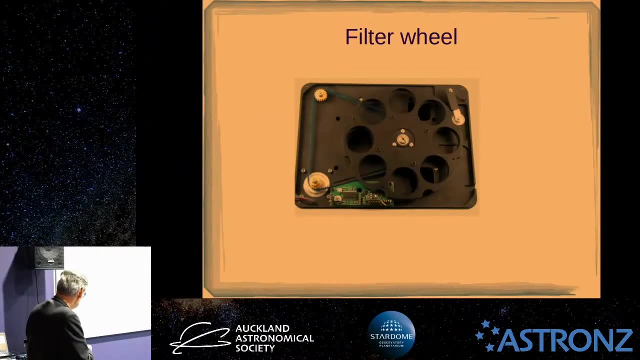 And a standard consumer camera will tend to block some of that out, So some people go to the trouble of getting the infrared cut filter removed. Probably voids your warranty Right if you're using one of these type of cameras or any kind of monochrome camera and you want to do color imaging. 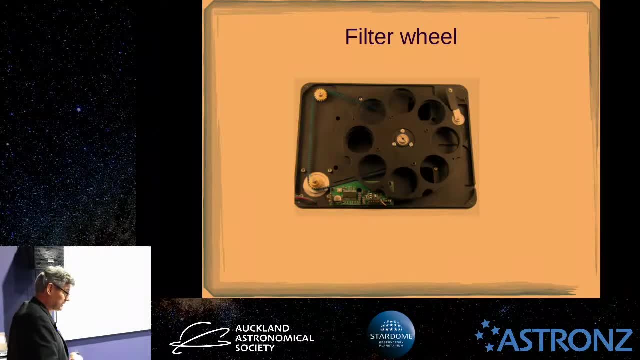 and you've seen the pretty pictures from the Hubble Space Telescope and so on- that has only monochrome camera or cameras- I believe there's more than one- But you use a filter wheel which is basically a holder of different kinds of filters. 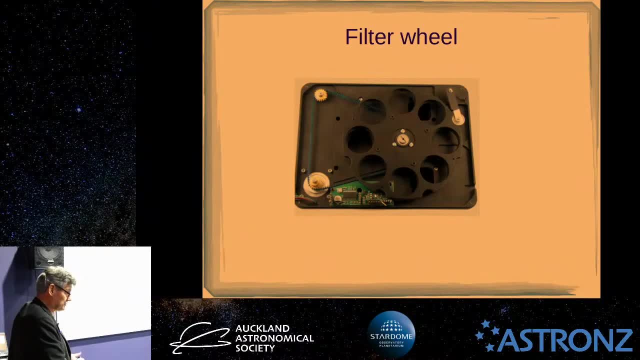 So you can. if you're just doing color imaging, you'd use a RGB and maybe a clear luminance filter And basically you have to take a separate exposures for each color and then you combine them to make a color image and post-processing. 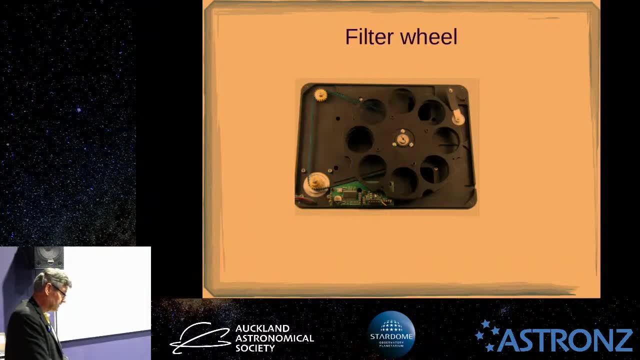 But filters are also used scientifically where you have a standard sort of band of light that you're interested in, or sometimes more than one, where you record each one. I think Chris Benton has talked about this for his talks on where you have B minus V. So you have a way. 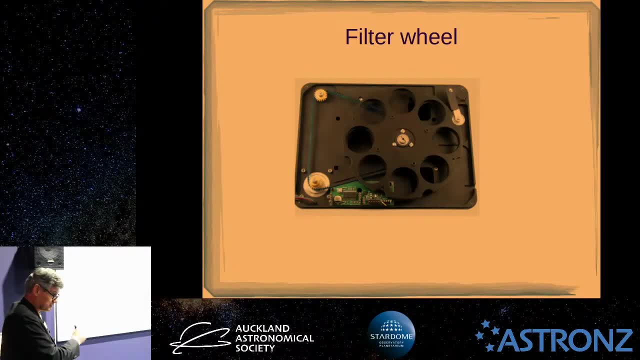 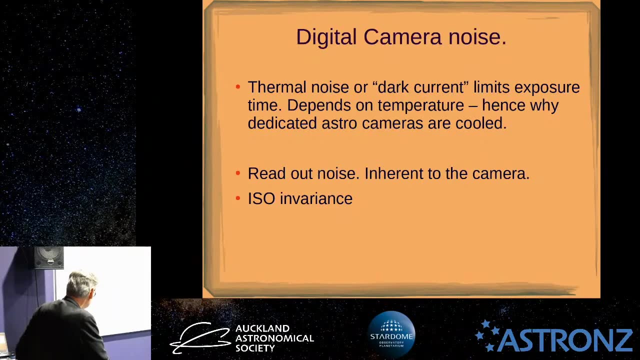 of measuring the colors of stars using the difference between what you measure and different filters. The bad thing about all these cameras? well, it's not bad, It's really inherent in them. And the longer your exposure is, the more noise that the camera starts recording. 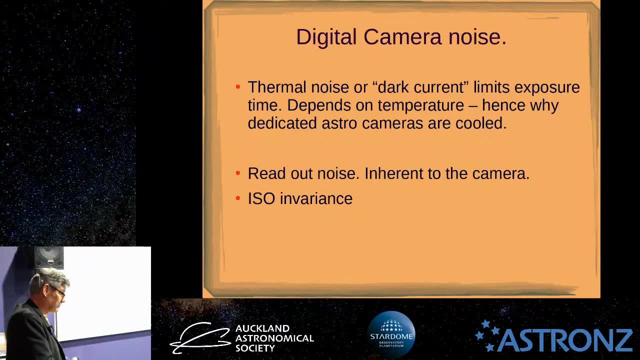 And you can't really do much about this. It's inherent in the way that you just get a bit of noise building up. The longer the exposure, the more it gets, But as long as your signal is a lot bigger than the noise, 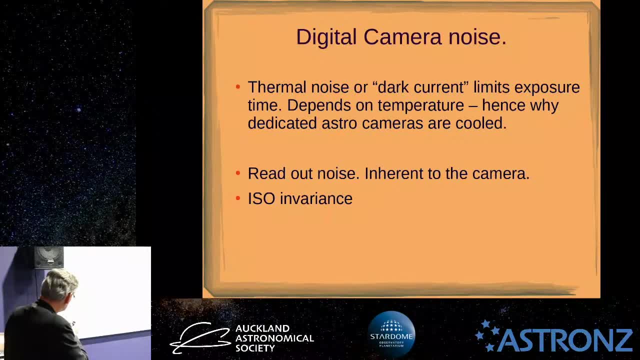 you're generally OK And you can see that the amount of noise whoops. did I go the wrong way? Yes, I did. The noise depends on not only how long your exposure time is, but also on the ambient temperature. So some of these cameras, and this one included. 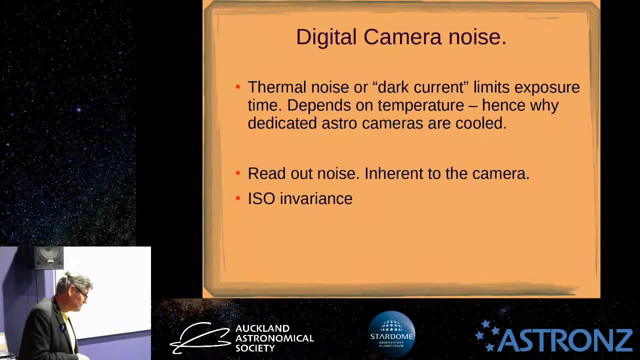 has got a refrigeration mechanism built in, So you do your imaging well, with the sensor cooled well below 0.. What's this one Grant, Go down to minus 40, or It can go down to at least minus 35.. 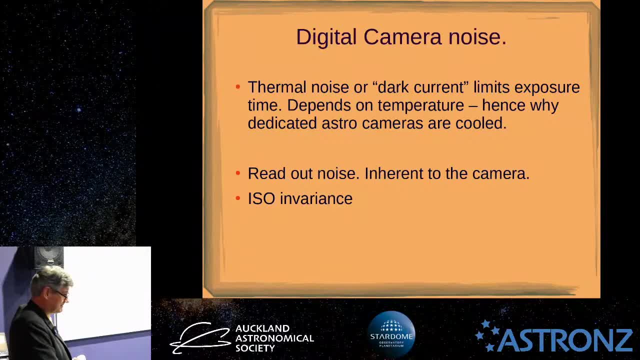 But maybe not an orphan, Something like that, Right? But so you usually choose the temperature you can get every day at any rate of the year. So we use minus 20 on the other one, Right, So it's a temperature delta you get. 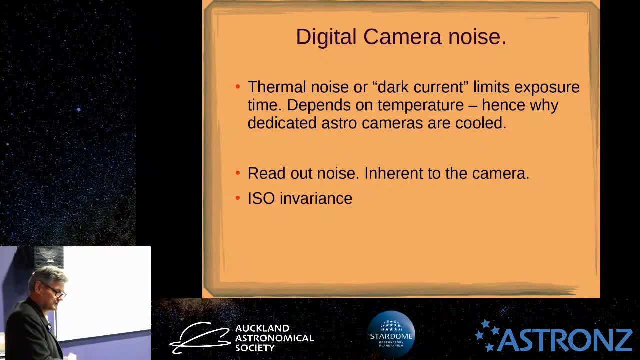 So normally they'll cool to, say, 30 degrees below whatever the ambient temperature, Right? So by doing that you get a lot less of this thermal noise, or sometimes called dark noise or dark current. So there's another kind of noise when you actually get the data. 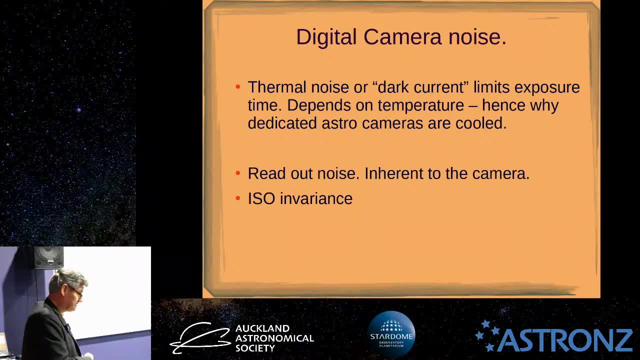 out of the chart. But there's electronic circuitry involved in doing that on either the CCD cameras or CMOS ones, And that itself, actually reading the chip, introduces some noise And as you see there that's inherent to the camera. So it depends on the design of the chip and the electronics. 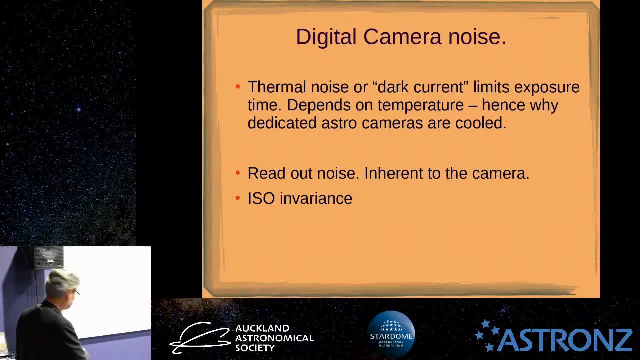 attached to it, what amount of readout noise you get. So I just put another note there about iso and variance. OK, OK, Because this is a kind of a silly thing that has been carried over from the old film days where you bought film of a particular iso. 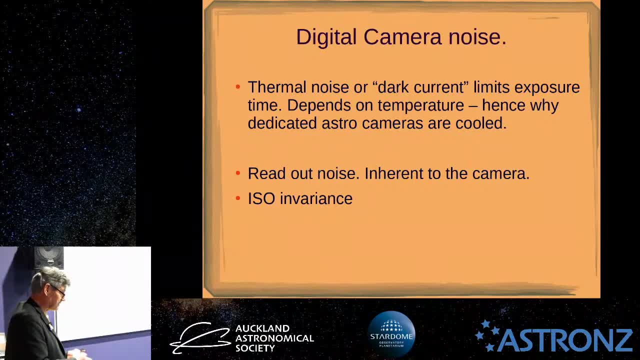 like a 400 iso film or a 100 iso. The 100 iso was less sensitive but the images you got out of it would be less grainy. The 400 will have a bit more grain in the image but you could take much shorter exposures. 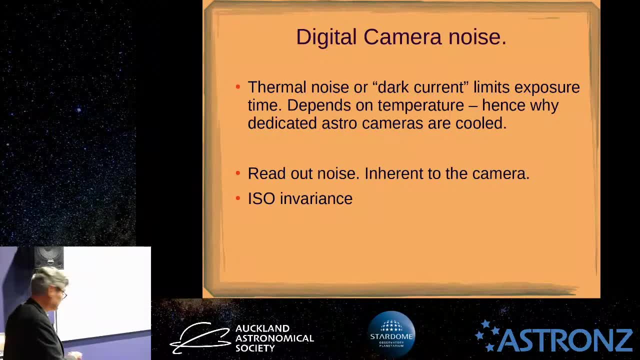 OK, OK, OK, OK, I'm going to do another. I'll cut the roll results footage of the Z reversal. OK, Great, OK, And if measures are running, I'll do that. You got the reference, OK. 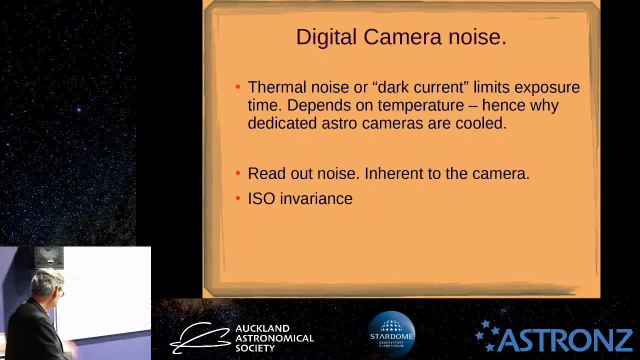 OK, OK, That's like a zero degree. He was a wyddo, OK, Yeah, OK, OK, Good, That's really cool. So, compared to asibergold, you want more surface color, but how are you allowing that cutoff to run discussion? 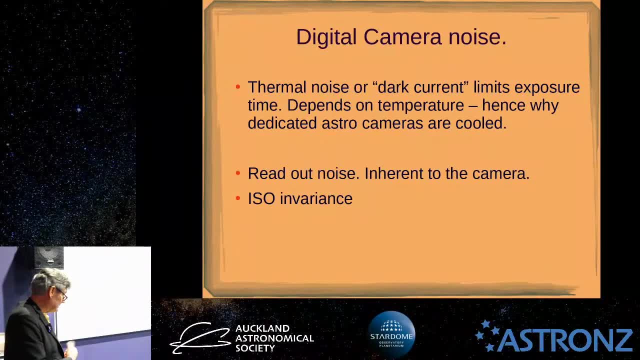 what amount of amplification to use. And basically, iso-invariance means that those amplifiers are linear, which they're not, But they are getting much better these days. So a really modern mirrorless camera or DSLR will do much better in this area. 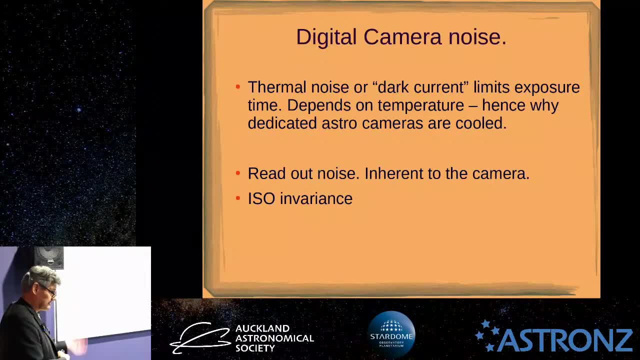 So there's not really a difference between taking a 100-iso picture in 1800.. If you stretch it in post, if it's iso-invariant, you'll get the same actual signal-to-noise ratio. So it's purely artificial. 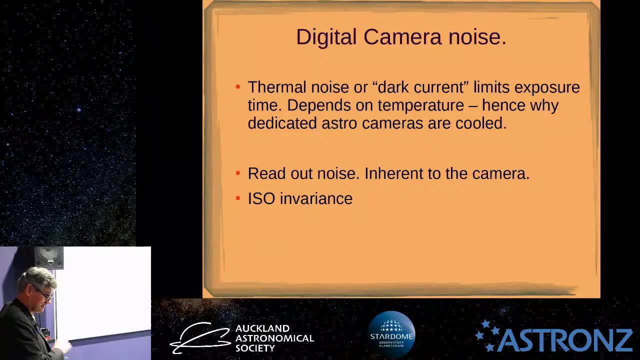 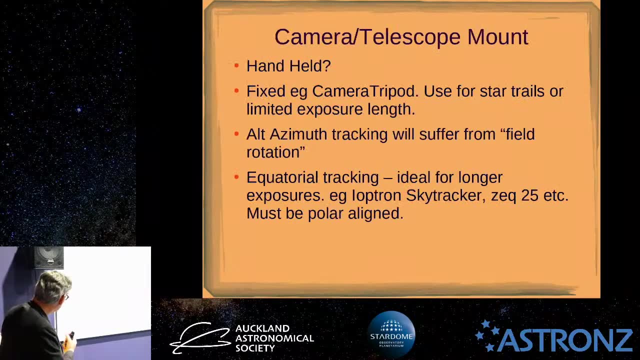 But some of the older cameras- higher iso, the amplifiers were generating a lot more noise. So it just depends on what system you've got Right. so you've got to have some way to attach your your camera or mount it. 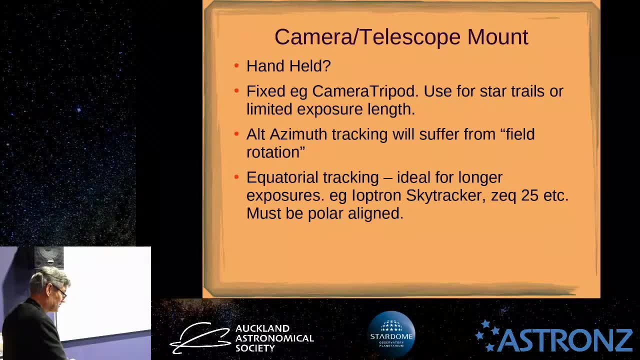 You could try handheld. It might be okay for bright objects like the moon or for some skyscapes where things are quite bright and you've got, maybe, image stabilisation in your camera and lens, But usually you would use a tripod at least. And this is just a camera, an ordinary camera and lens. 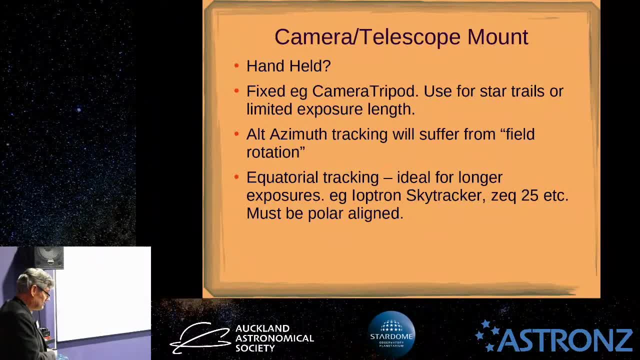 sitting on a tripod And you see these, a lot of these skyscape images, and some of them are fantastic-looking images. That's basically all they've done, And I think this year's judge, Babak Tafreshi, who judged the Harry Williams trophy this year. 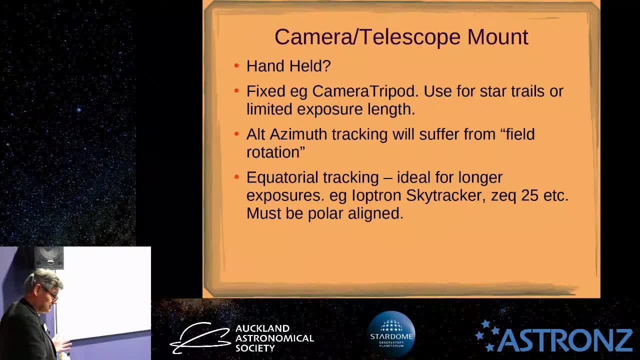 he actually prefers. this kind of single-shot image Puts a lot of limitations on what you can do, but he's not keen on a lot of processing, So I thought that was quite interesting. Obviously, with deep-sky images, you haven't got any choice. 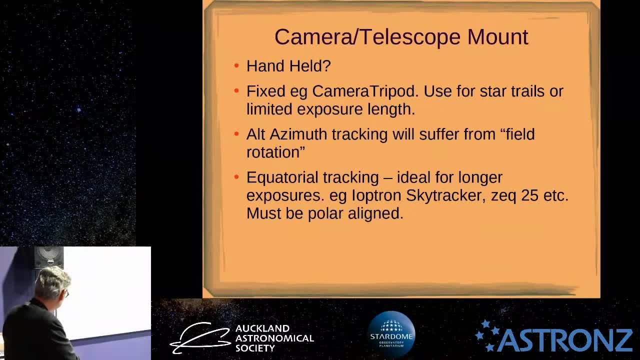 but to do a lot of processing and I'll explain that later. You know you can put it on a mount that's tracking the sky. So if you're following stars or planets and your mount is tracking, that's fine. if it's an alt-azimuth mount. 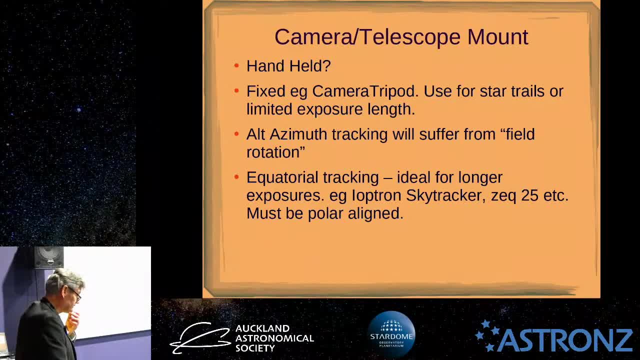 but you get an effect called rotation of field or field rotation, And I'll explain that a bit further on the next slide or two. And I'll explain that a bit further on the next slide or two. And I'll explain that a bit further on the next slide or two. 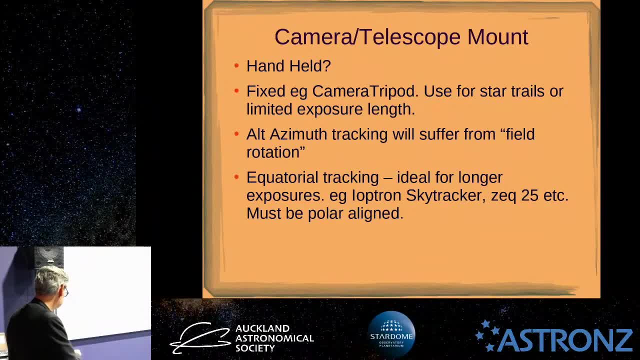 Or you can do equatorial tracking, Or you can do equatorial tracking And you can get fairly small, portable ones, like the Iotron SkyTracker, Maybe a slightly bigger mount ZEQ25.. And they are lined up with the Celestial Pole. 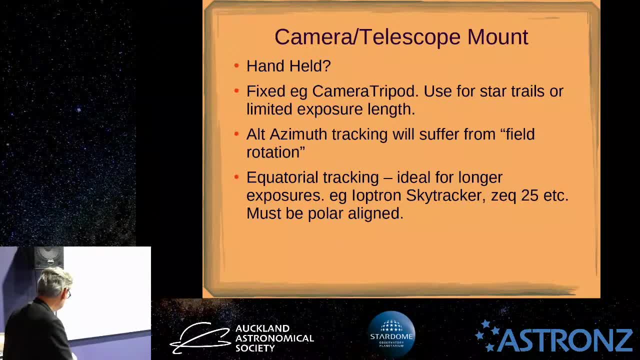 And I think we've sort of covered this before. but basically you only have to rotate the mount in right ascension, So it's basically rotating around the line of the sky. So it's basically rotating around the line through the pole, So to follow the stars, and it stops them streaking. 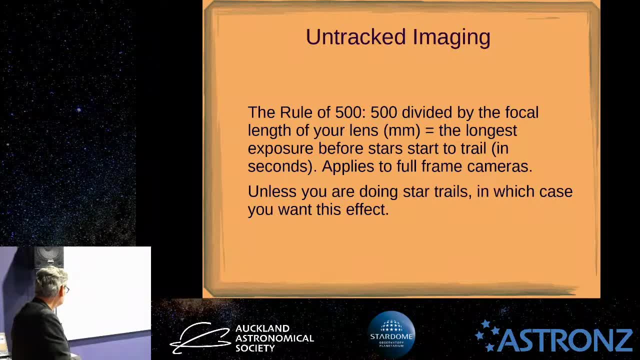 So if you're doing untracked imaging, there's a so-called rule of 500.. It's a little bit dubious because it depends on the camera and the pixel size and the size of the format of the camera- Generally a full-frame camera, you can get away with this. 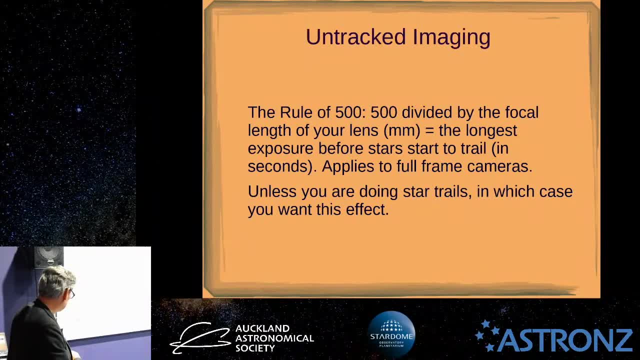 You basically divide the focal length of your lens into 500. And that gives you the longest exposure you can get before you'll see the movement of the stars in the picture. But if the pixels are really small, like some of the cameras, you can get, 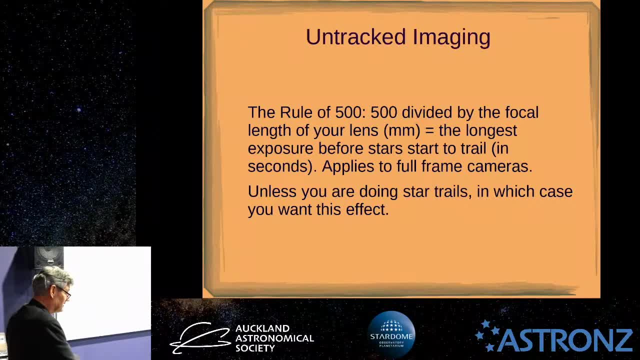 like 40, 50 megapixel cameras, you will see the trailing a lot earlier because the pixels are really small. So treat that formula with a grain of salt. So you'll probably have to. you'll have to experiment, But yeah, you can get quite good images. 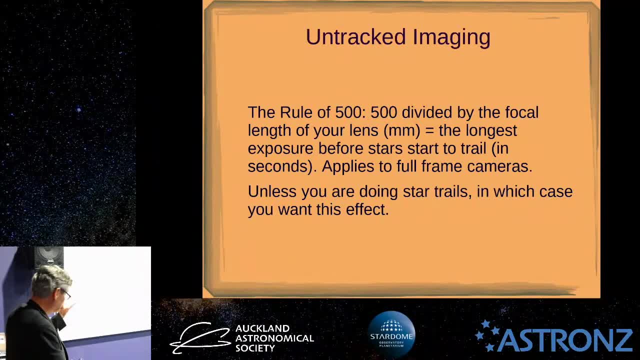 just a fixed camera on a tripod, as long as you don't go too long to where you start to see the stars streaking. So sometimes, though, you might want the stars to streak, and this is called a star trail image- I'm sure you've seen these- where you actually have the stars. 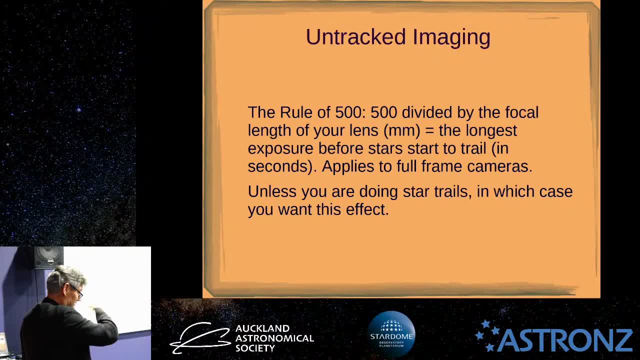 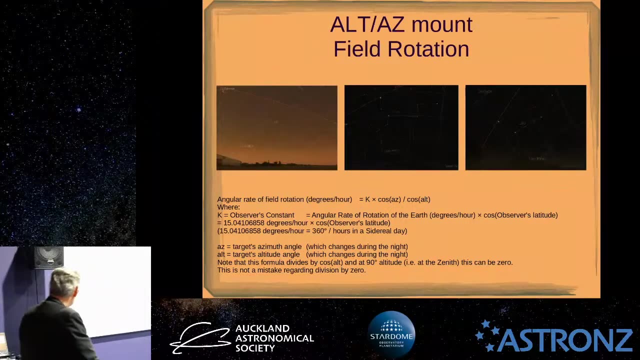 showing streaks across the sky Going around the South or the North Celestial Pole, and they can be quite effective as well. Okay, I mentioned about Altair's rotation of field. I don't know that those pictures show up that well. 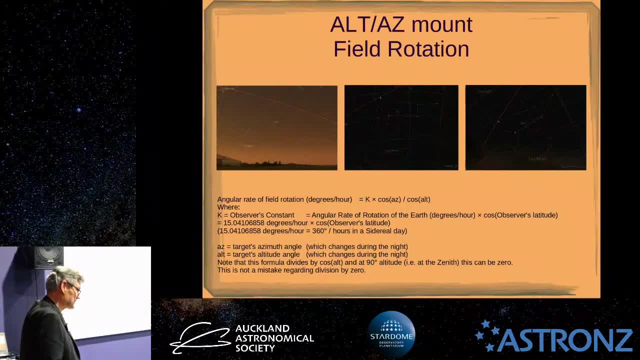 so I won't use those. They're a bit dark on the screen there. If you imagine- probably an easy way to imagine it- you've probably observed the Southern Cross In the winter. the cross is high like this and pointing towards the pole. 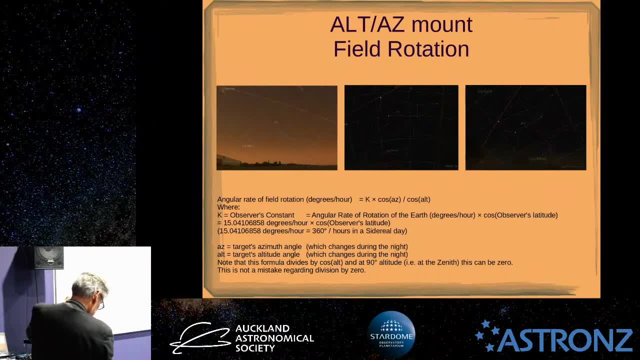 which is below the cross. Summer, the cross is below the pole and right down on the horizon in Auckland. But if you think about it, the cross down on the horizon is actually rotated from the one up here, So it's done a 180 degree turn. 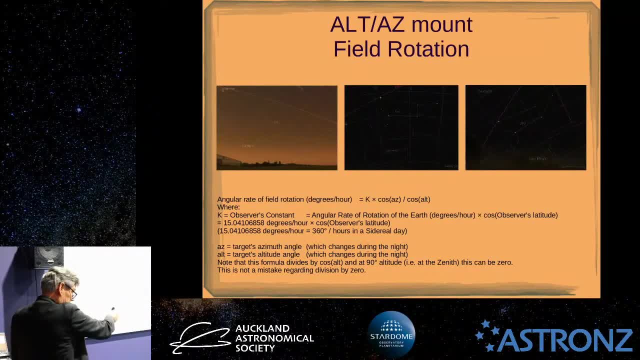 The Southern Cross is over here. It's rotated 90 degrees from what it was when it's high in the sky. If you were following that with an Altair's telescope, you'll actually see that rotation in the field that you're looking at. 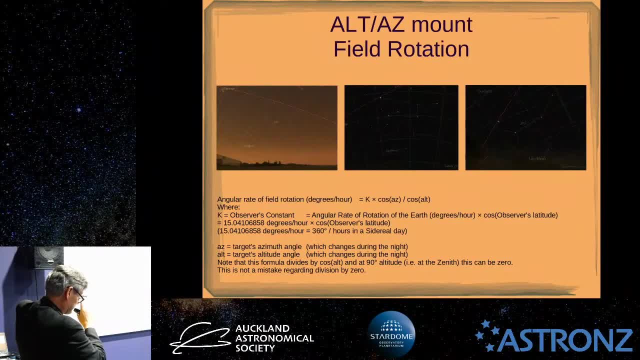 or the camera will see it, because the camera's in a fixed position. So what you end up within your picture, you'll see the stars starting to streak in little circles within the field of view of the camera. So the fix for that is: you can get silly. 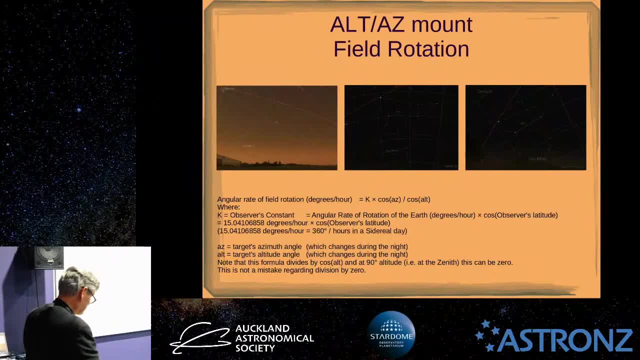 and buy a device that rotates the camera the opposite way. And that's what the big professional observatories do, because a lot of their really big telescopes are on Altair's mounts And down below there. oops, go back that formula there. 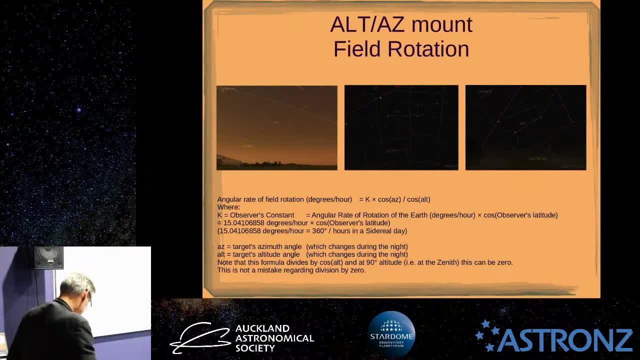 if I press the right button. I'm not sure what's happened to my pointer. maybe the battery's dying on me. Oh, there it is. You can calculate that the cosine of the azimuth divided by the cosine of the altitude times what's called the observer's constant. 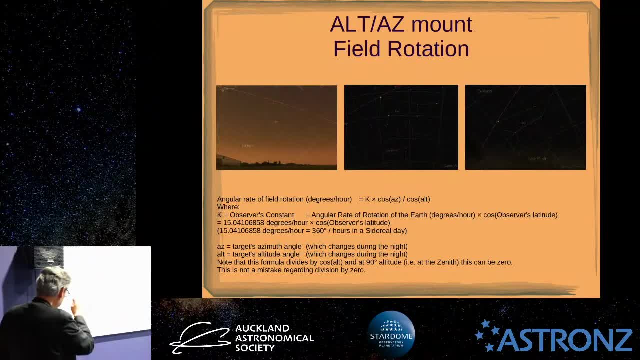 And you wouldn't really ever bother with that. but if you wanted to build a field derotator, you have to use that formula to figure out how to counteract the rotation of the stars in your picture. So you don't want to do that really. 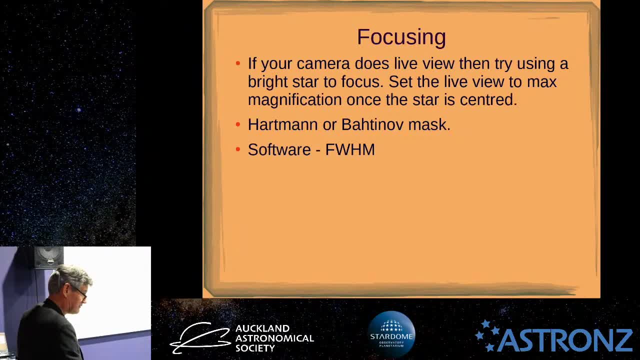 so you use an equatorial mount that's aligned with the pole. It's a lot easier for amateurs, Although that's a trick in itself doing accurate polar alignment. That's for another session. I'm sure Steve will talk about that sometime. 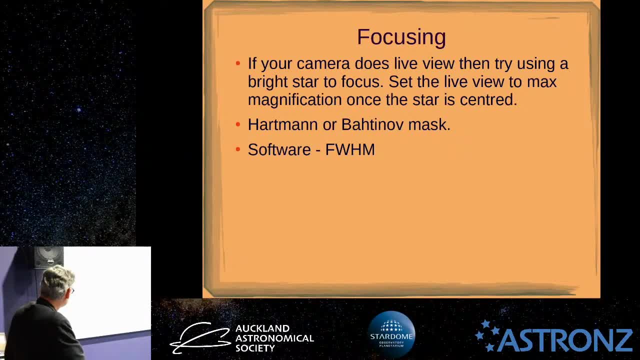 Right. The other trick you have to worry about is focusing. So with a DSLR or mirrorless camera, the ideal thing is if you can get a live view on the screen. on the back, you aim it at a fairly bright star. 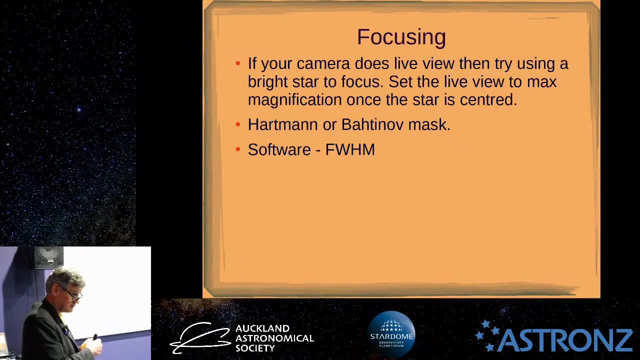 and you can normally magnify the live view either five or ten times. Start it at five times manually focus to get the star to as small a point as you can, Then go to ten times magnification and do it again. It kind of works okay. 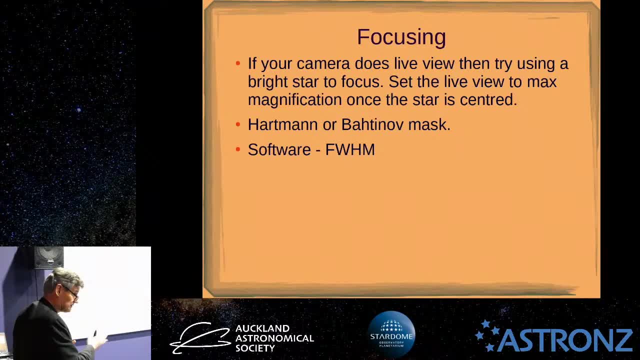 It definitely works well for skyscapes. with a wide angle lens On a telescope it's so-so, as I think Albert found out last week on the Zeiss, It's pretty hard to do it. Another way you can do it is a Hartmann or Battenhove mask. 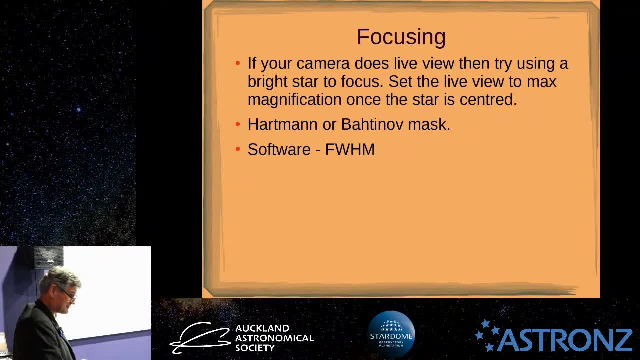 I find particularly the Battenhove mask quite fascinating. I'll show you a little gif of that in a minute. And the other way is to use software and you look for what's called the full width at half maximum And what that is. 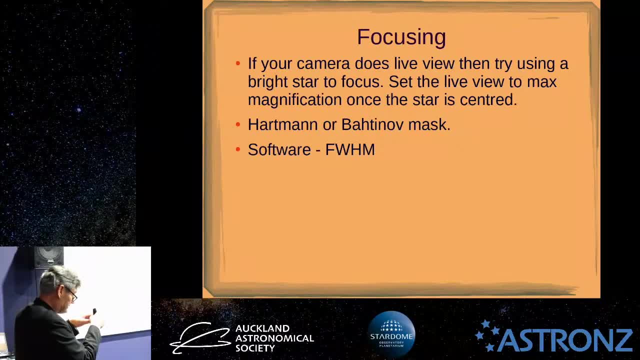 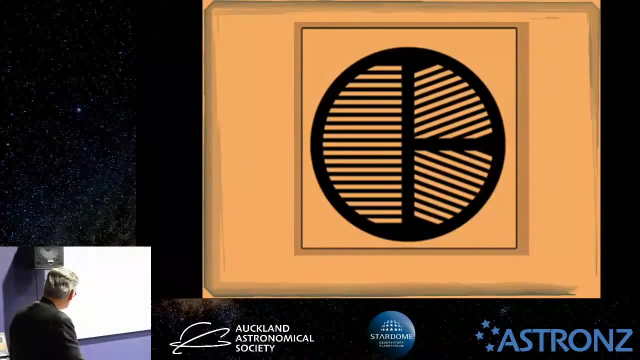 is basically in the software. you inspect the image coming off the camera and star images will come up with a peak like that, And the idea is you want that peak to be as narrow as you can get it. So let's have a look. That's a Battenhove mask. 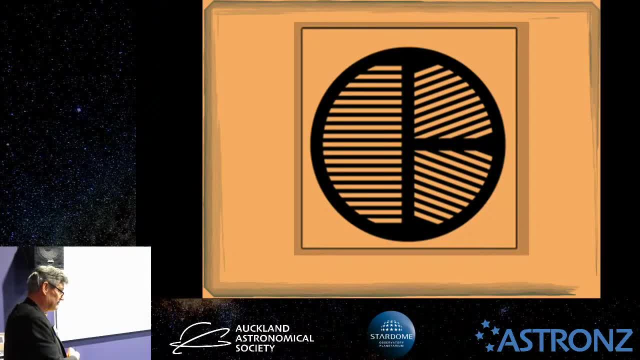 So there are actually patterns you can get for these off the internet to make them yourself, for different size masks, and you can print them and then cut them out on a sheet of hard material. So they kind of look a bit like a strange looking drain cover. 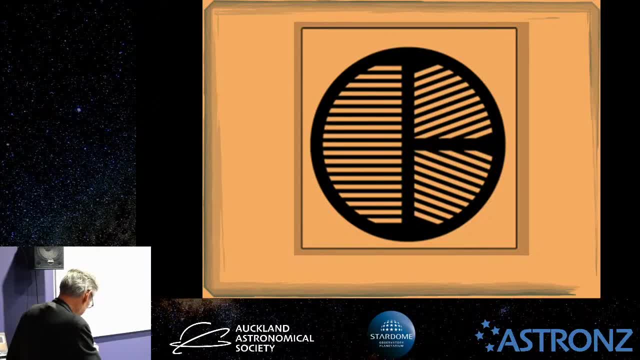 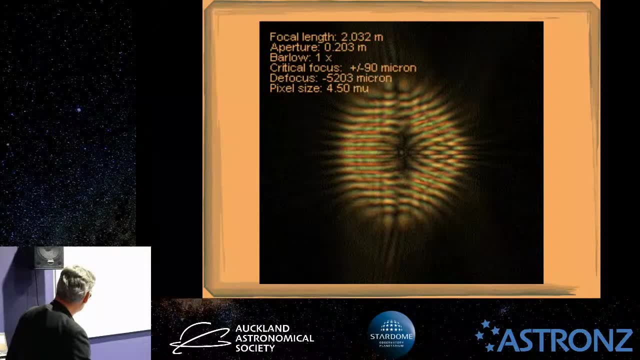 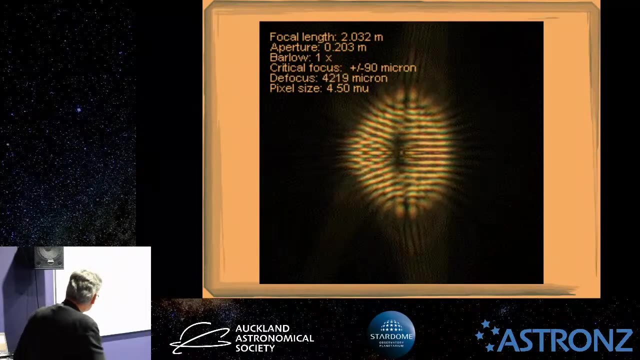 But this is what they do. I guess Battenhove must have been pretty clever to work this out. This is a Battenhove mask in action. as you're moving the focuser in and out on either side of focus, It might be a little bit fast to see. 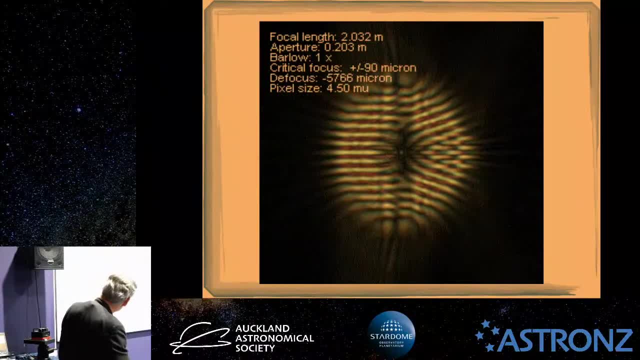 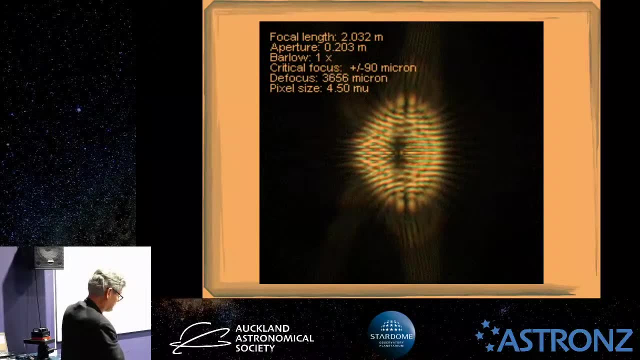 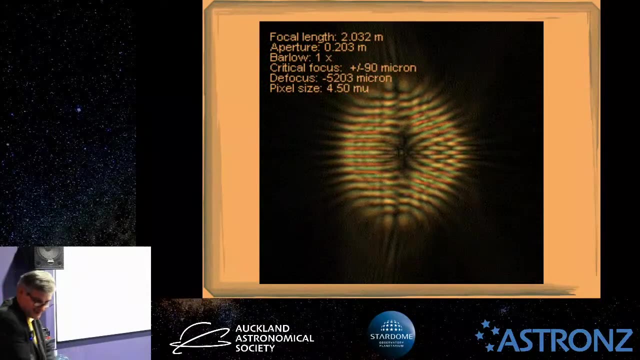 but if you look, then you start seeing the diffraction spikes When the central spike is dead, in the centre of the two crossing ones. that's when you've got really good focus. So anyone ever use one of these? Oh, Steve. 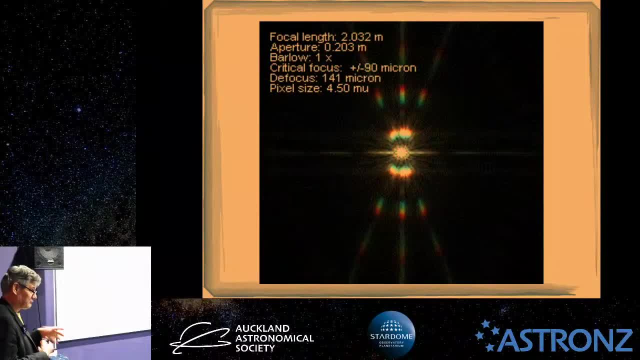 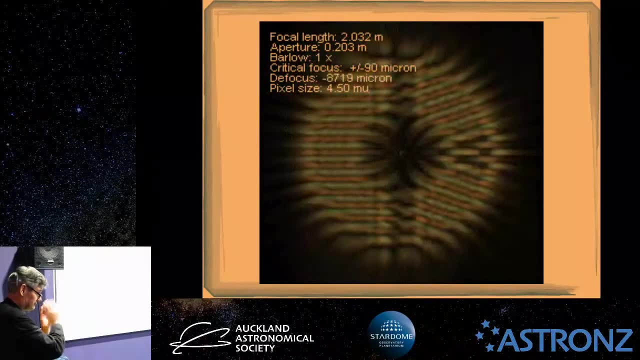 The two Steves have used one. So if you've got a camera lens, you can use this. You put it over the front of the camera lens. Same with a telescope, But you have to make one for the right size for your objective. 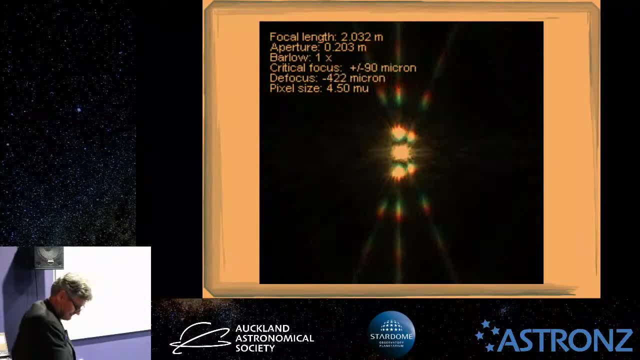 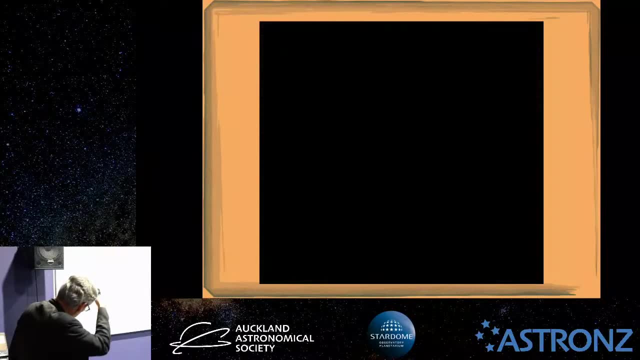 The axe you're looking for in that crossing line that moves left and right as you focus. Yeah, if you look carefully, you'll see that you want to wait till it moves to the dead centre of the two. Yeah, so you've got an axe. 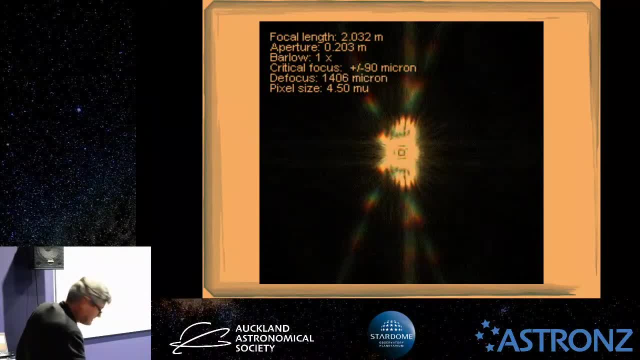 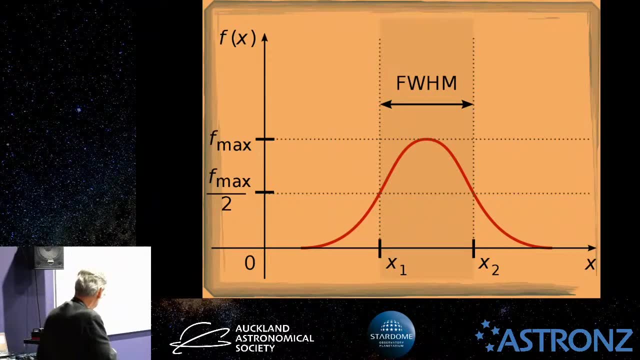 and you've got that line in the middle there. That's when it's focused, And this is what I was talking about with full width, half maximum. So the idea is that you want to, And often, um, there's some software programmes. 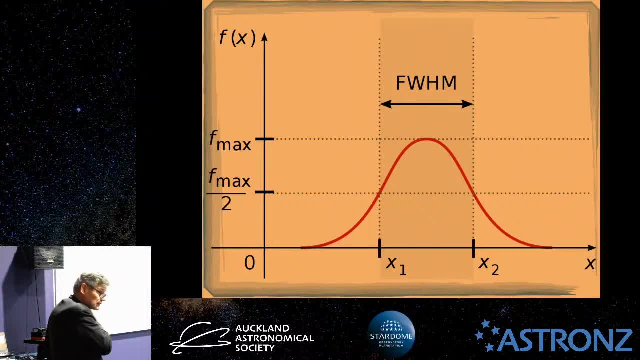 that will control cameras and so on. Like for DSLR, there's one called Backyard EOS, which you plug into your camera and you can control it from a laptop And it will monitor a star for you and it will measure the distance between X1 and X2.. 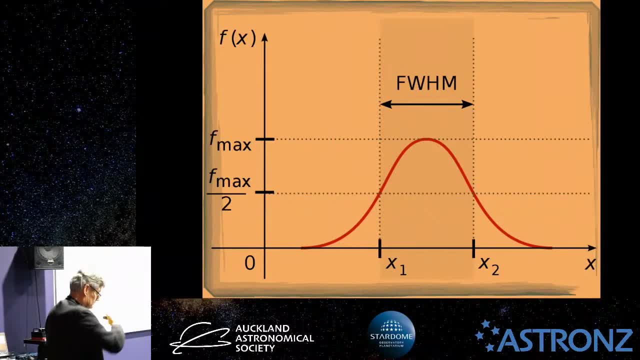 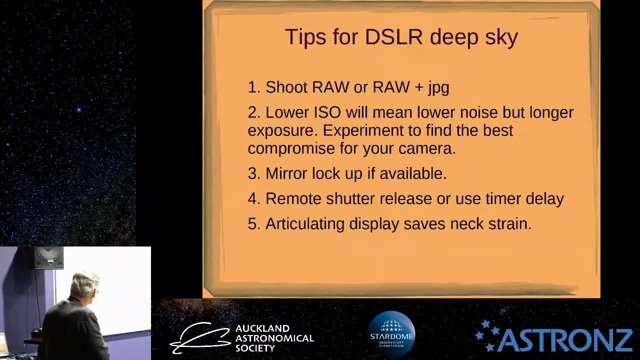 And the idea is, the absolute number doesn't matter, but you dial the focus until that number is a minimum Right? Just some basic tips. Probably, if you're doing DSLR photography, you're best to shoot in RAW rather than JPEG images. 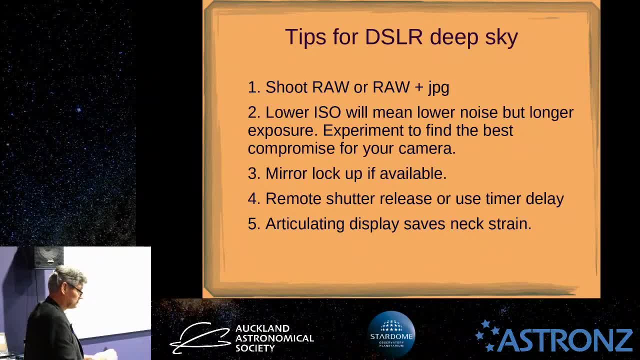 The RAW data out of the camera holds a lot more information and you can stretch it more and you can do frame calibration and things like that. And I'll just mention that shortly. Ideally with most cameras you want a lower ISO because you get a lower amount. 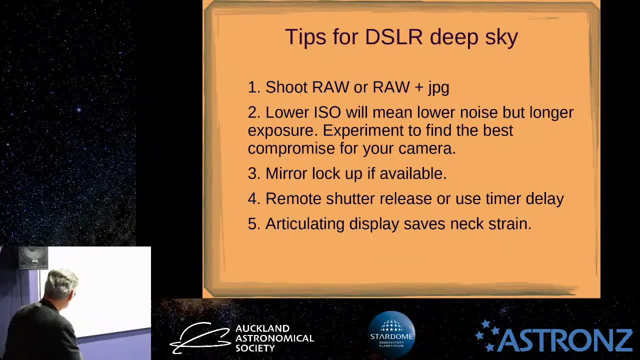 of amplification noise from CMOS chips generally, But you've probably got to experiment to find winding up the ISO as high as you can get away with is good because it means you shorten your exposure time, but you don't want to start introducing a lot of noise. 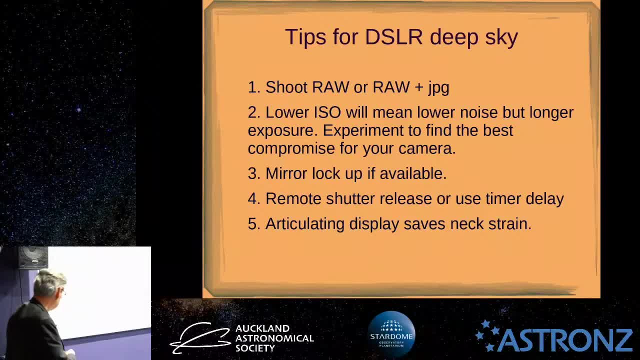 In a DSLR. if it's a a mirrorless one, you don't have to worry about this. but DSLR with a mirror, you want the mirror locked up. The reason for that is that if it flips off at the beginning of the exposure, 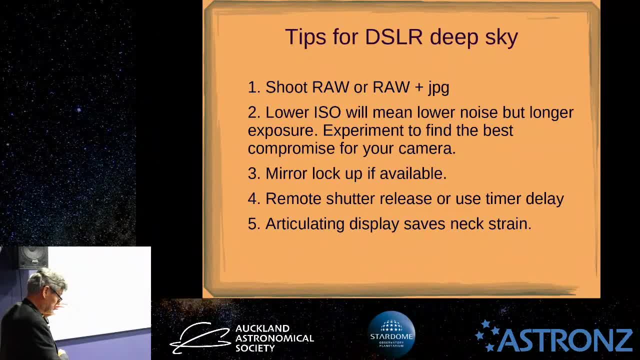 it actually will cause a little bit of vibration which can take a little bit of time to die out, and so you might get a little bit of shuddering going on in the image. You wouldn't notice that in daytime use of the thing when you're doing a 200th. 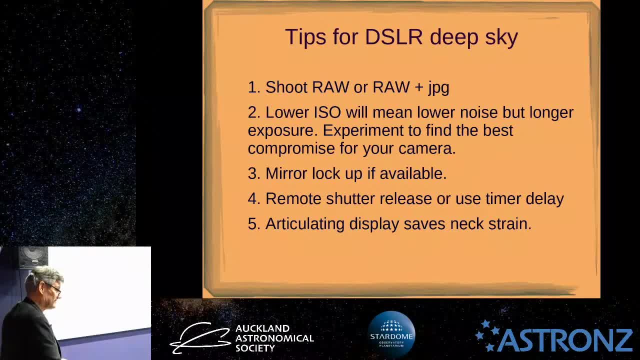 or a thousandth of a second because the shutter's open for such a short time. it doesn't matter if there's a bit of vibration from the shutter, And what you want to do is probably use a timer delay or a remote shutter so that again. 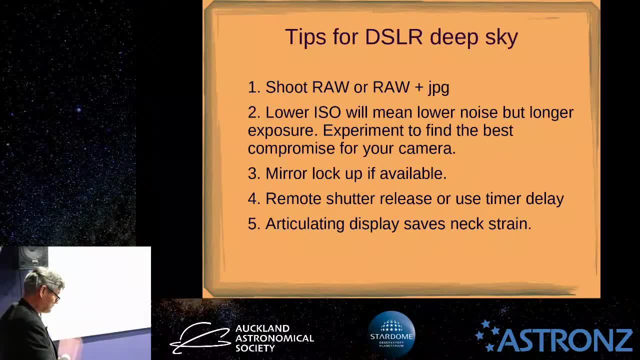 if you press the button on the camera you're going to cause it to shake, so use a remote Or most cameras. you can say wait 10 seconds and then take the shot, So that gives it time for any avoiding any vibrations. 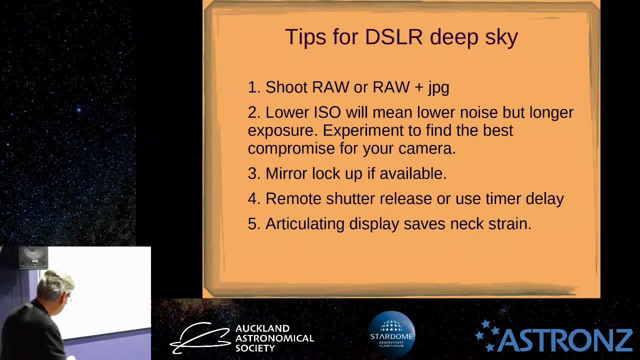 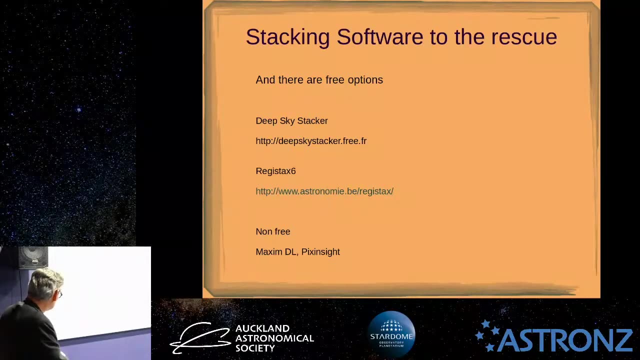 from your hand on the camera, And a lot of cameras have these articulating displays on the back, which are quite handy in certain positions to be able to see the live view without getting into a funny position Right. What we can do is take a whole series of images. 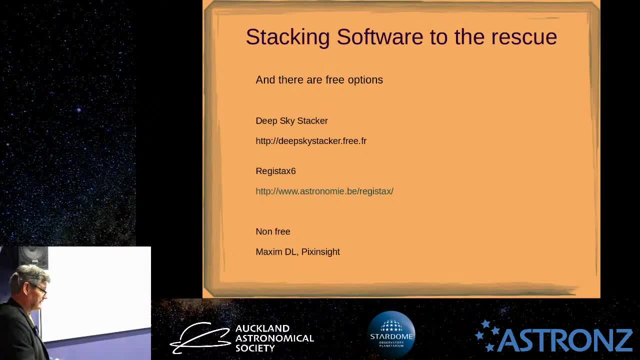 of your deep sky object and because of that thermal noise issue you can't take a one-hour exposure. The noise will just basically flood the thing eventually and you'll get totally useless data. So you have to find out how long an exposure you can get away with. 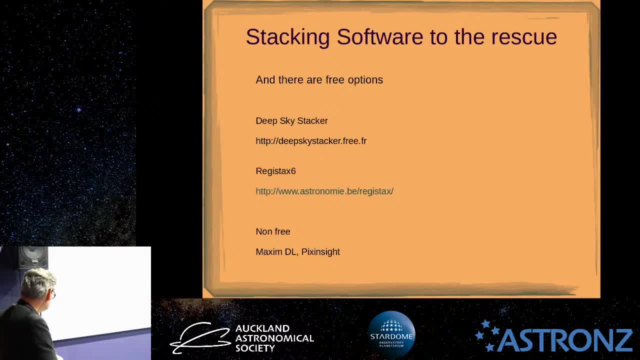 It'll depend on your camera, But the problem is that you may not capture the faint objects or enough detail in the faint objects. So what you do? you take lots and lots of images and you stack them together And there's some freeware programs. 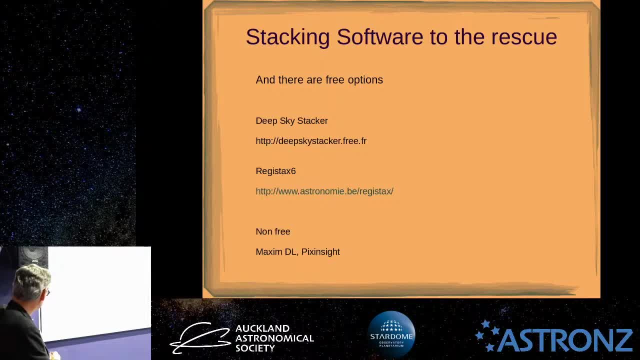 that will do this for you. There's some paid ones as well: Deep Sky Stacker, Registax 6.. Generally, Registax hasn't been updated since 2011.. No, so maybe not so good, but Right. 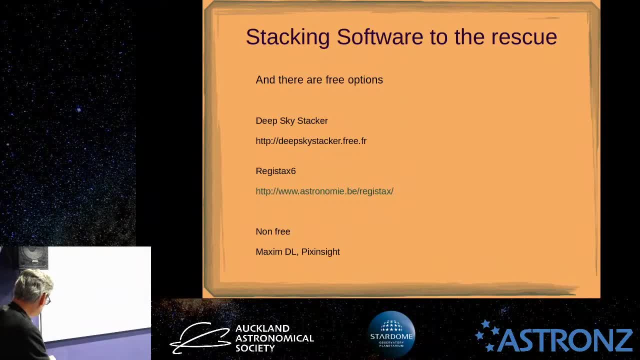 Right, OK. Yeah, Registax 6 was sort of more aimed at planetary imaging, And people used to say Deep Sky Stacker was the way to go for general deep sky shots. So yeah, AutoStack it too. I think it's called, isn't it? 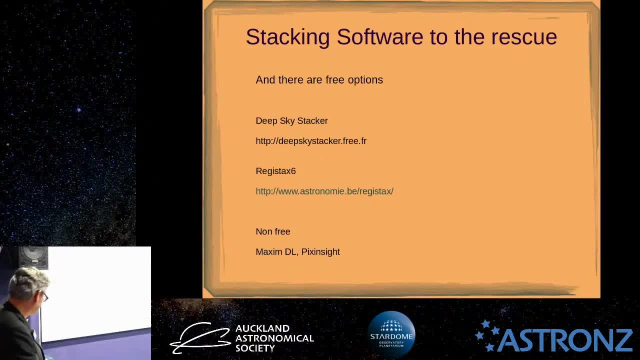 Yeah, 3 now. Oh, they've got a new version. OK, Registax 6 did have some really good sharpening. It's still used for the way it does the sharpening. All right, Right, so you. 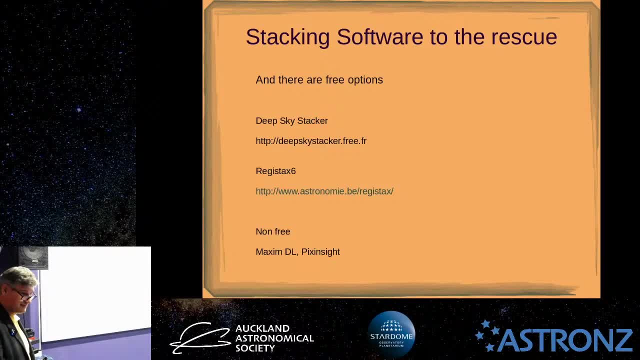 Yeah, I think people use both. They do the stacking in AutoStack at 3 now and then use Registax 6 to do some final image sharpening. It's much better than the sharpening you get in Photoshop or GIMP or any of those programs. 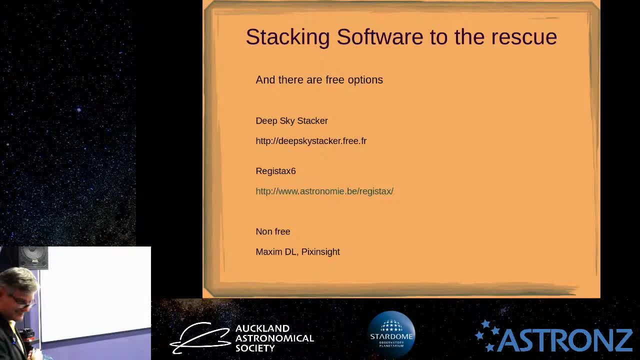 It's a bit magical the way it works. actually, I've seen the thing in action. These programs at the bottom- Maxim DL- not only does image acquisition, it does all sorts of other things as well, a lot more than just Deep Sky Stacker does. 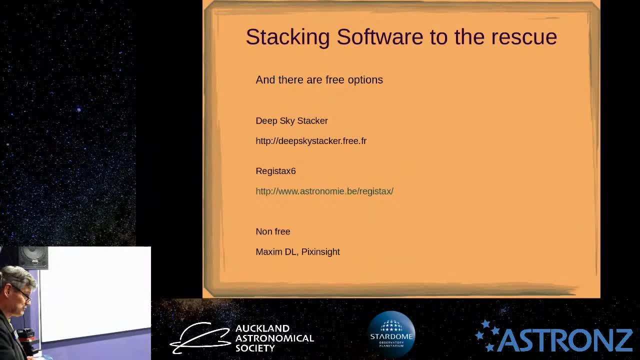 and PixInsight has a really high-end image processing program. I know people like Rolf Olsen- some of you may know his work users and other people- but unfortunately they're not free programs, And particularly PixInsight I understand. I've never used it myself. 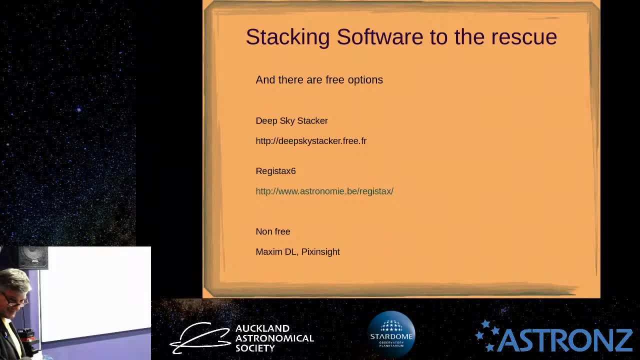 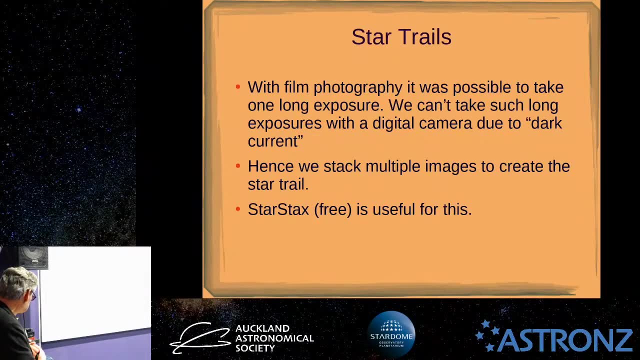 has a really long learning curve. Have you tried it, Steve? No, Right. So I talked about star trails before, So there's, Basically, you take, say, a whole bunch of 2- or 3-minute exposures where the stars are straight. 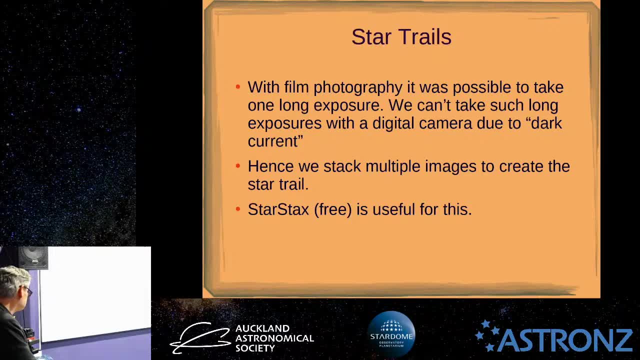 but you want to join them together. So a good program for that is called Star Stacks. it's free. There was another one called- A guy in Hong Kong wrote it, I've forgotten his name- Secutor, which does this as well as similar things. 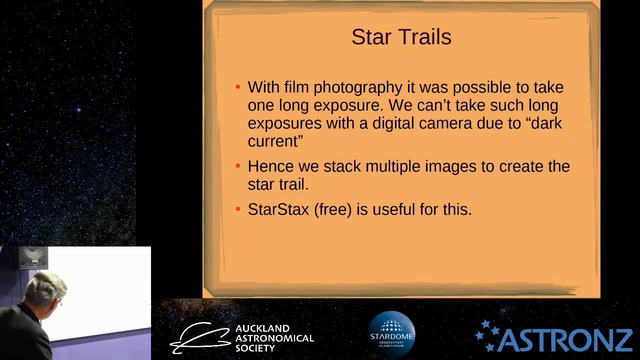 to Deep Sky Stacker. But I found Star Stacks is quite good because it cheats, because when you do a whole lot of these star trails images, there's a tiny gap between each trail, and Star Stacks is a cheat mode where it'll actually fill in the gaps for you. 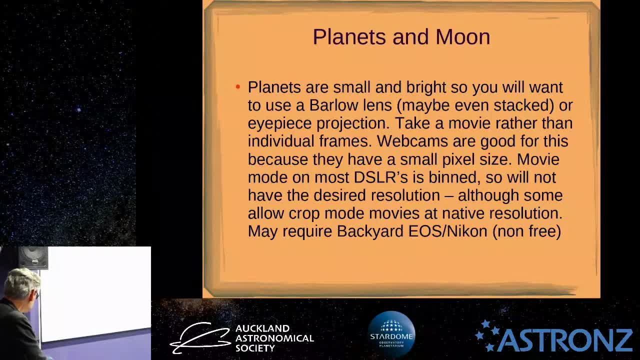 OK, So I mentioned before that planets are small and bright, so for most telescopes you'll want to use a Barlow lens. You wouldn't need to on the Zeiss upstairs if you were using that for planetary imaging, because it's already got a really long focal length. 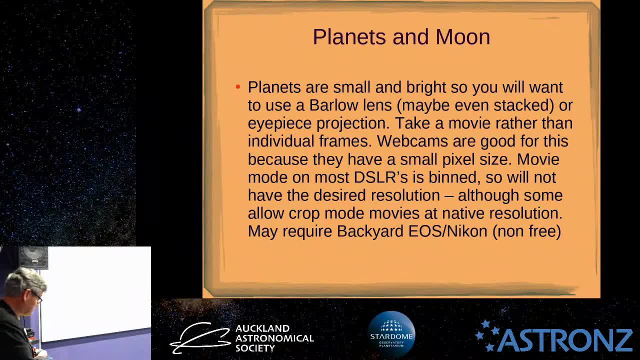 that prime focus of 6.6.. 6.6 meters. So it's probably pretty good for planetary imaging as it is, But other telescopes, the planets, will be too small on the camera sensor to get nice images. Generally, most DLSR's movie mode 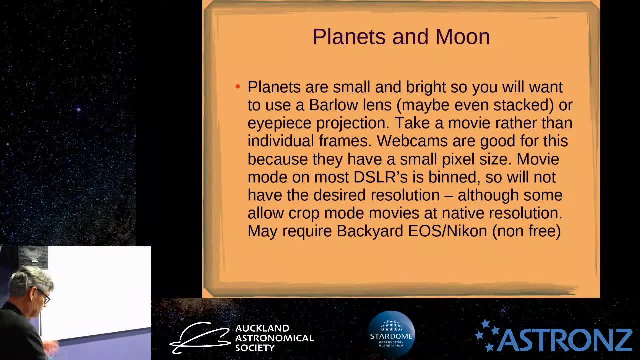 has been from the main sensor, but some of the new mirrorless ones you can do for even 8K imaging so you might be able to use those for planetary imaging. But you'll get really huge files of the movies that come out of those. 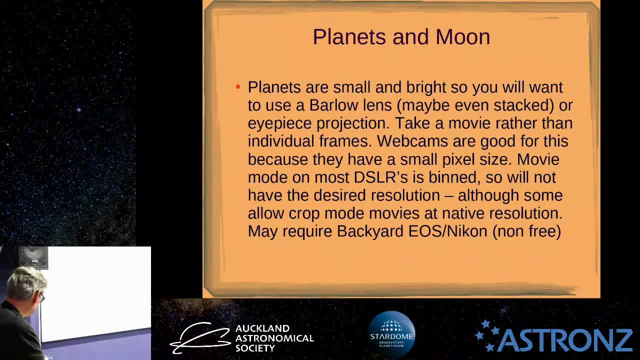 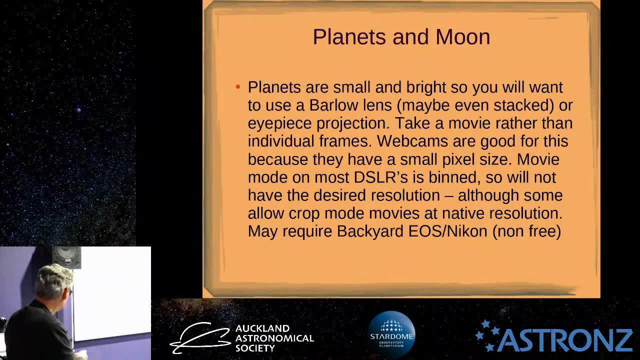 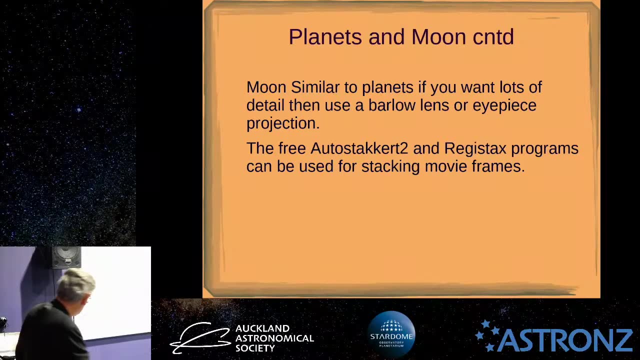 And you can for controlling your camera to do this sort of capturing. there's some programs like Backyard EOS or Backyard Nissan. Nikon are quite good, And actually I mentioned AutoStacker 2.. I should update that slide now that AutoStacker 3 is out. 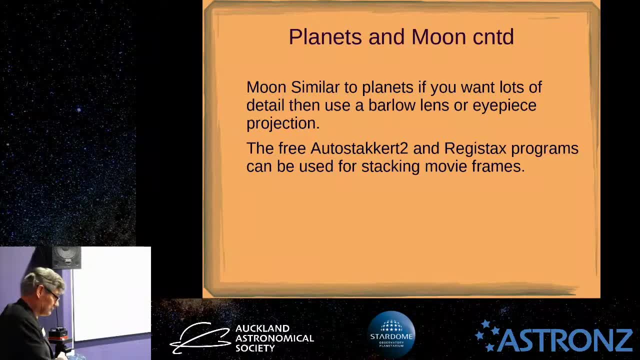 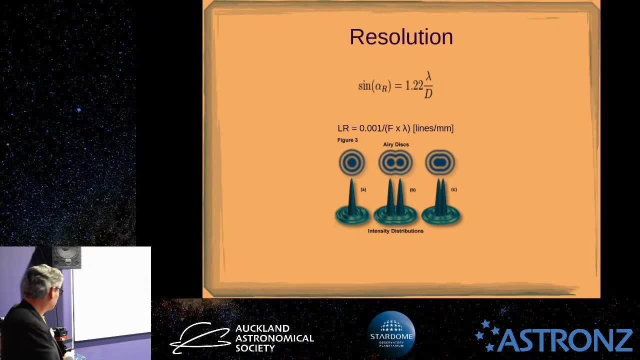 So you can use these programs for stacking, basically, movies of the planets. So how are we going? time-wise, Not too bad. Just a little thing about resolution. We talked about camera resolution. You can think, oh, if I have a smaller pixel. 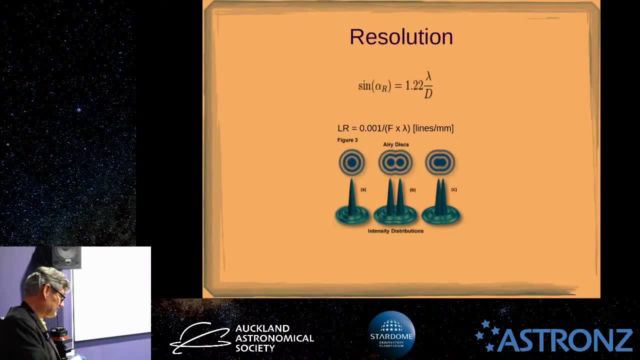 I can see more detail. Well, that isn't really the case. There's two reasons: because of this resolution. So what? this is telling you this here, the big D is the aperture of the telescope, So you're dividing lambda as the wavelength of the light. 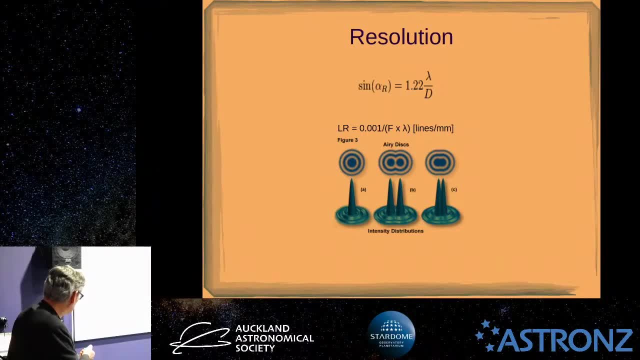 So obviously the wavelength of blue light is smaller, So you're going to get slightly better resolution in blue than in red. And you divide by the aperture of your telescope and that will tell you the sign of the angle that you can resolve on the sky. 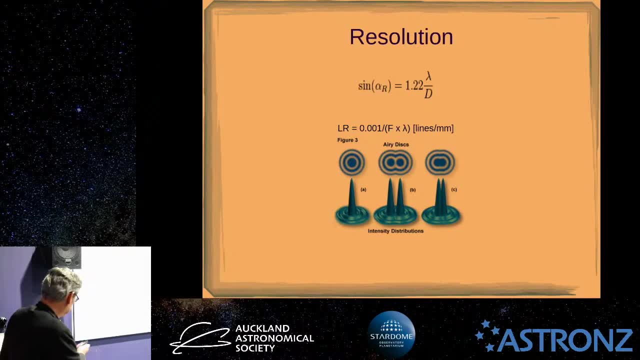 So it doesn't matter what the focal length of the telescope is. It's purely a function of how big the mirror or objective lens is. So you can scale the image up using a Barlow, but you may actually get no more resolution. 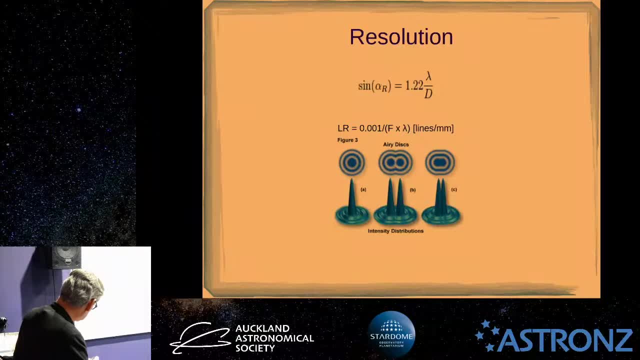 And this sort of explains what the image of a star forms in focus in the Erie disk And it shows like a three-dimensional graph of that, And so those two would be considered well resolved, because you can distinguish the two peaks Once you're getting down to here. 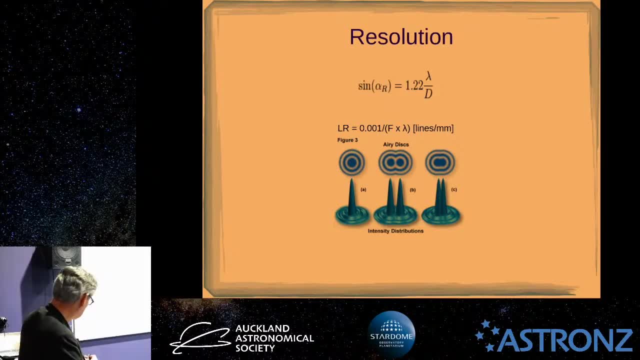 the two stars getting too close together are really hard to resolve. So this is sort of an empirical formula. I think Lord Valley figured this out originally or published something on this. So the other thing that's counting against you if you have a really big mirror. 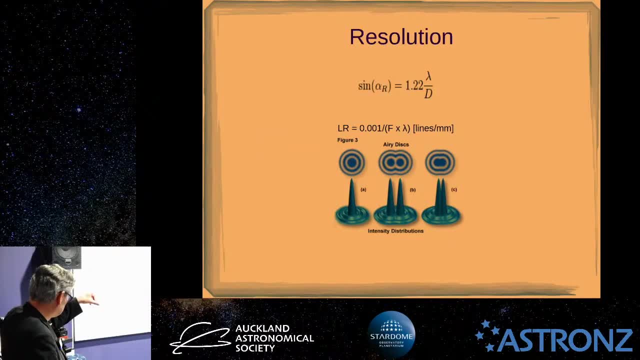 like the Zeiss or other big telescope. you might have a really good sub-arctic and resolving power of the optical system, But you're never going to achieve that in reality because the atmosphere is going to act against you In Auckland, I think, on the best nights. 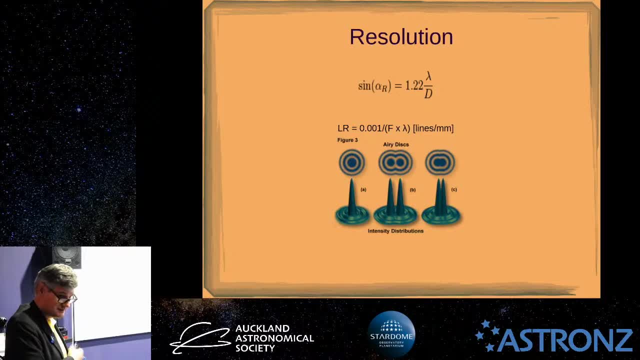 you get something like an arc second down to an arc second, but that's on a really good night, So if you're resolving a lot less than that, it's probably not going to do you much good. You get into what's called oversampling. 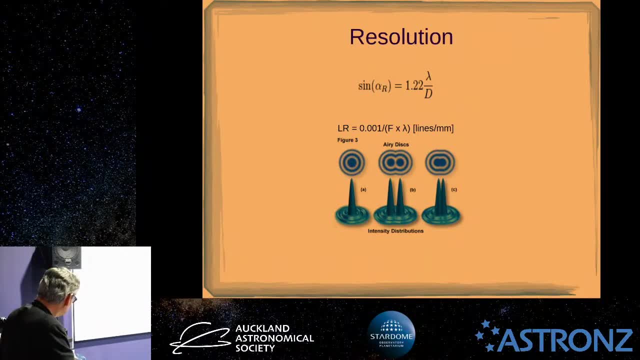 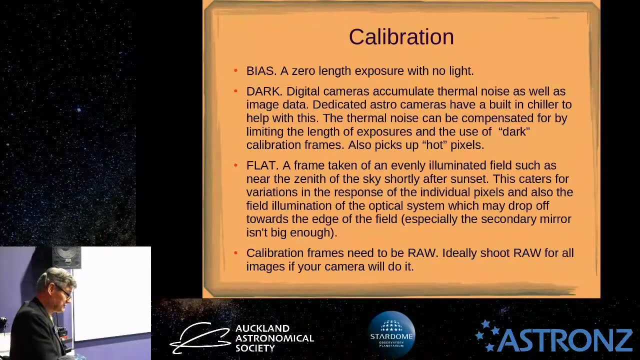 So another topic is calibration of the images. Talked about stacking. Well, there's a way we can deal with some of these faults. So the first one is a bias frame. You basically take a bunch of exposures of zero length for the fastest exposure that your camera will do. 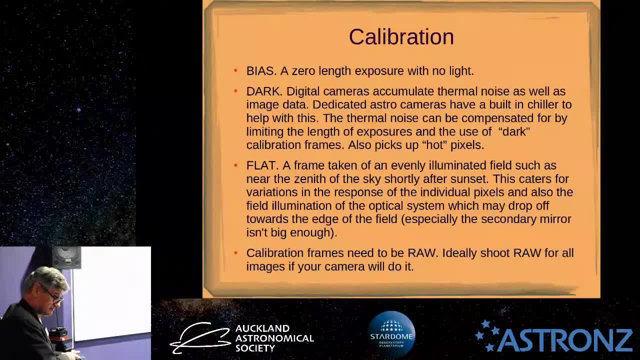 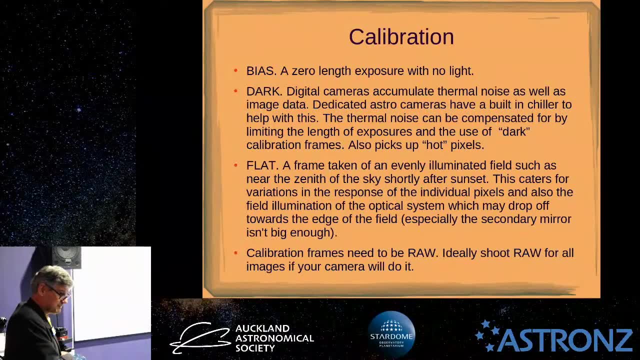 Lens cap on or light completely blocked out of the camera, And basically what that's measuring is the read noise of the camera. So you save those frames- read noise for your camera. then you can take what are called dark frames. So if you were imaging at 30 second exposures, 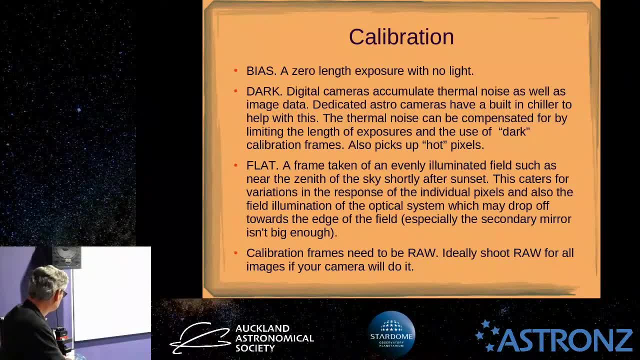 of an object in the night sky. what you do is then you take a whole bunch of what are called dark images, same settings in the camera, same exposure length, So you're just going with the lens cap on or the light blocked off. 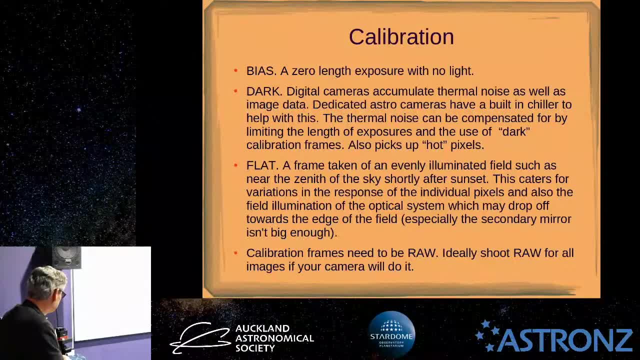 from getting into the camera And you're basically measuring the thermal noise. So this has to be done at the same temperature that you took your light images at, So it's no good doing these dark images during the day, when it's a lot warmer, of course. 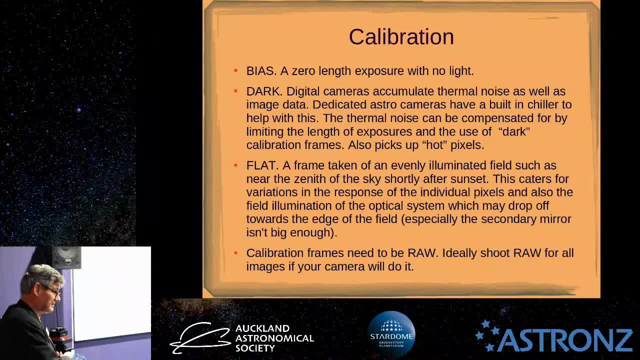 because it'll be measuring a lot more noise than you'd get at night when it's cooler And cameras themselves generate internal heat. DSLRs do, But you're better to do the dark frames at the same angle, At the same ambient conditions as the light frames. 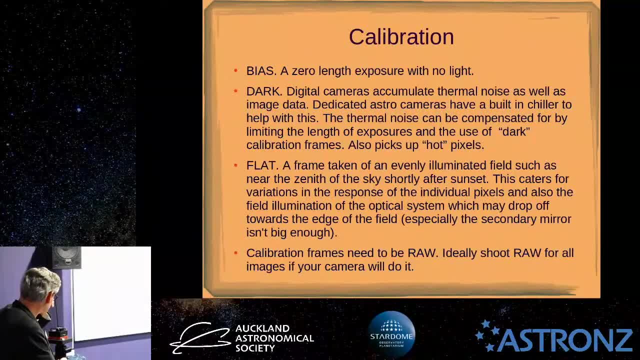 So they'll be more useful. So dark frames also picks up some errors in your chart, One of them called a hot pixel, which means it just reads out maximum value all the time. So most cameras will have a pixel or a few pixels that'll have that fault in them. 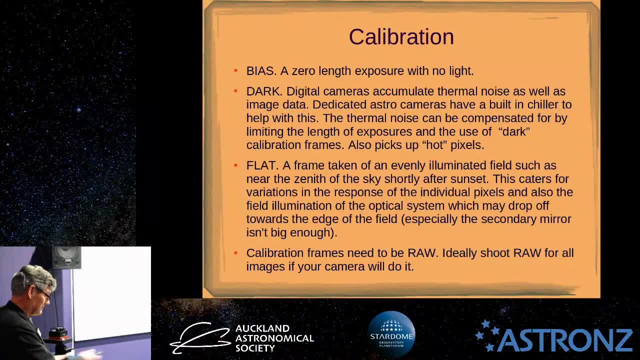 So the dark frames will detect those, obviously, because you suddenly have a really bright pixel in the middle of a picture that was taken with no light. You get an opposite to that actually is a dead pixel that reads nothing, no matter what light is exposed on it. 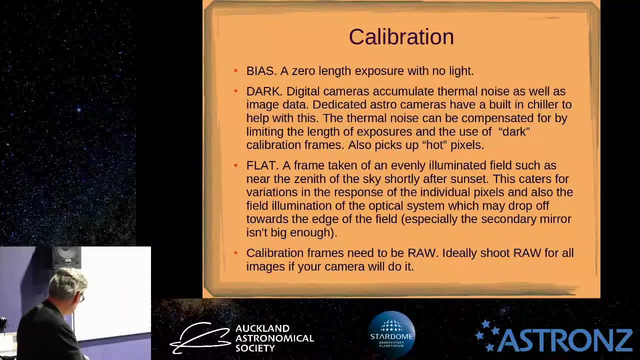 So you take another type of calibration frame that's called a flat, And often the most convenient way to do this. take a picture of the twilight sky before the stars are getting there, And this is picking up a few variations, Generally a lens or telescope. 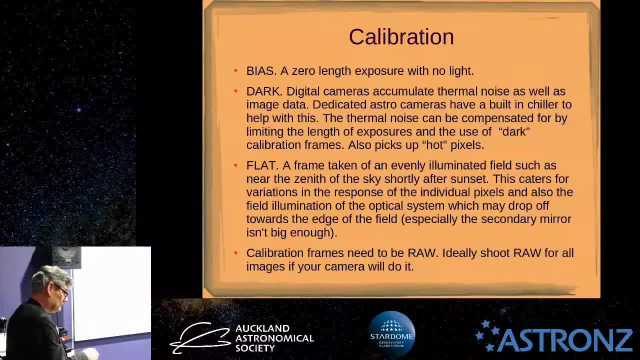 it may not be fully illuminating the field of the camera. So you've heard of vignetting, maybe, where the corners of the picture are a little bit dimmer than in the centre of the frame. So this is actually measuring that. 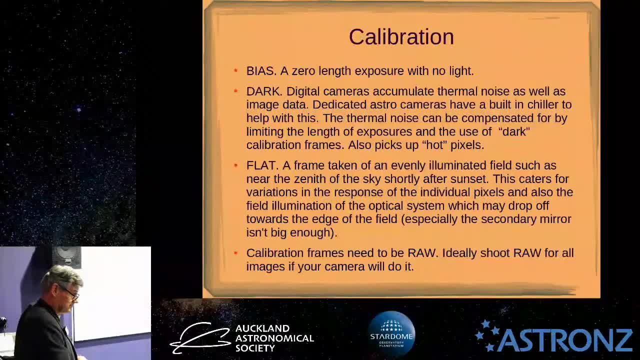 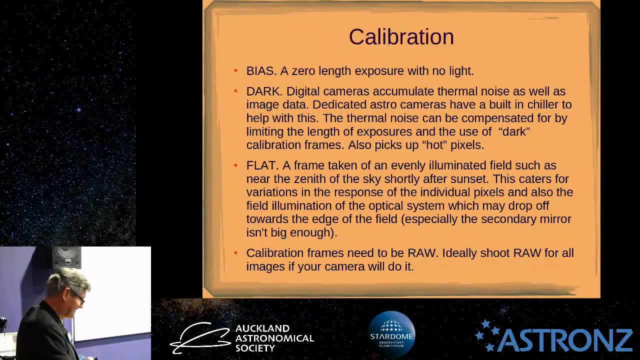 and it's also measuring any dirt. Maybe that's causing what are called dust doughnuts- I don't know if you've heard of those in the image. So that's what these flats are taken for. So they're basically used to take out the flaws. 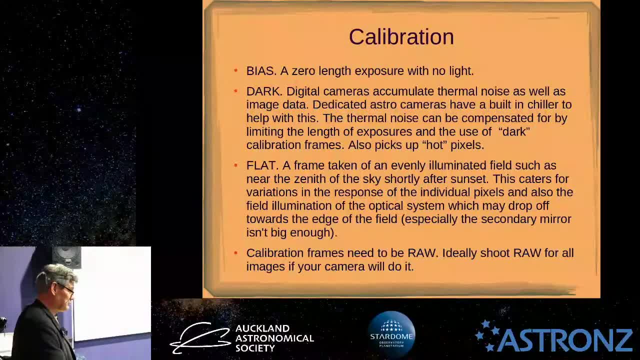 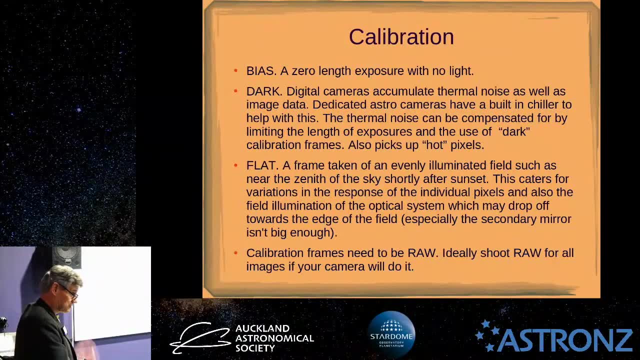 in the pictures that you're taking to get the best possible result And your programmes like Deep Sky Stacker understands what to do with these images. You just say: here are my darks, here are my flats, here are my bias frames. 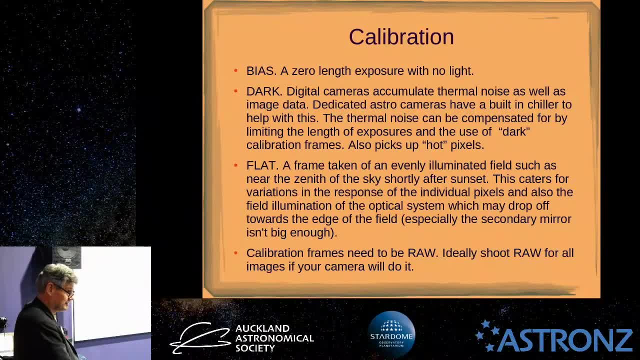 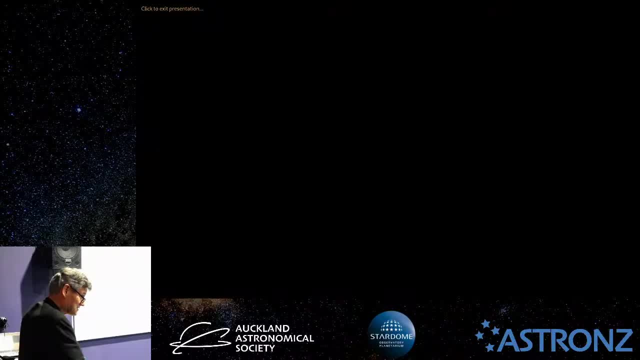 You don't have to use them, but it will improve the quality of the final image, And that's all I'm going to talk about today. So, if anyone's got any questions, A comment about the RAW files, The most important thing about shooting in RAW. 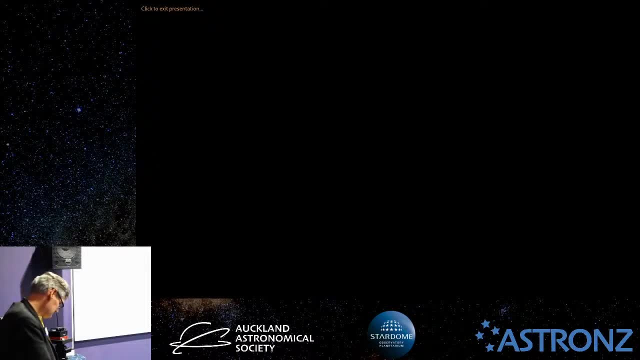 is partly. the camera doesn't do any processing, so you get the image as the sensor captured it. but the most important thing is the amount of different light levels that your camera captures. So if you convert an image to a JPEG, then each pixel in each of the colours. 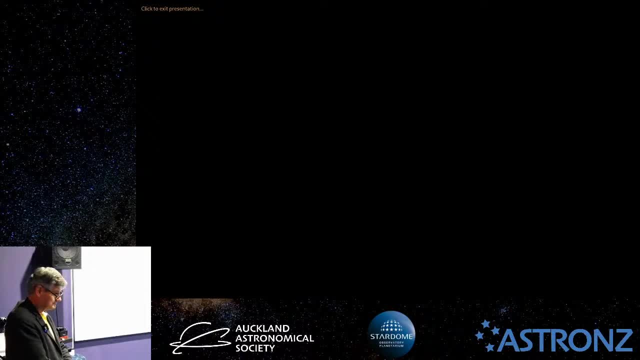 has only got 256 different brightnesses it can be at, So you've got something very bright in the frame, like a star, and something very dark in the background. There's only 256 even distributions of bright and dark that can be captured. 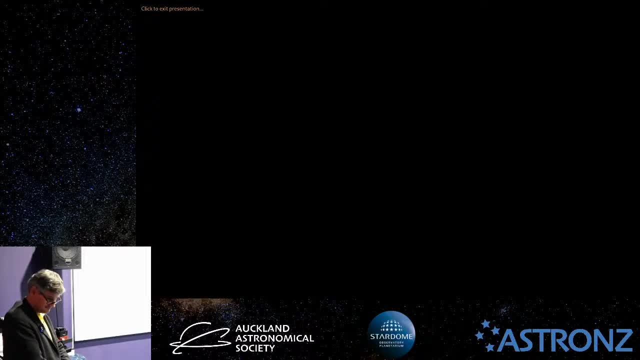 If you're shooting in RAW, then you've got, depending on your camera, 12,, 14, or 16 bit, which is up to 65,000 different levels. So that's the measurement of the difference between the faintest thing you can see in the picture. 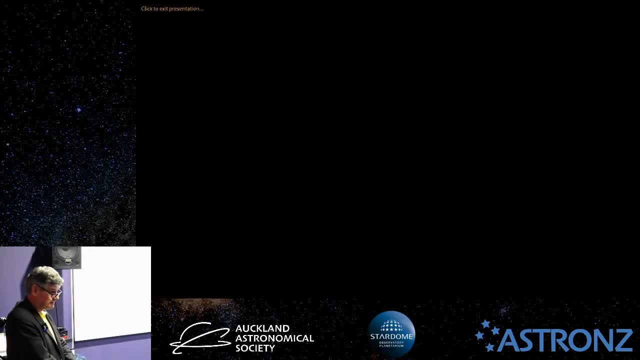 and the brightest thing you can see. So yeah, I think some of the newer cameras are using a new format which is sort of like JPG, but it has a higher dynamic range- HEIV or something or something like that, But there's not many programmes that'll deal with it. 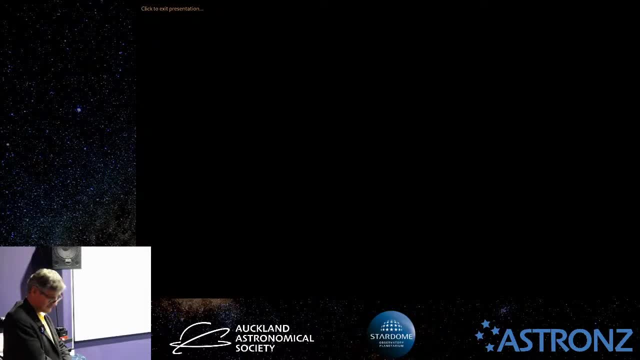 so it's a bit of an issue. So you're looking at the bit depth. 8-bit is not much good. that's what the JPEGs are, but RAW is going to be 12,, 14, or 16.. 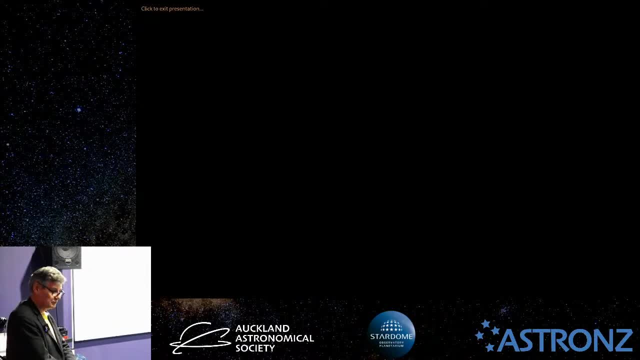 Yeah, it's fine for publishing your pictures on the internet on a website or something, but if you want to have really high-quality images there, you need more bits of colour depth. If you want to learn a lot more about this, you can join the Astrophotography group. 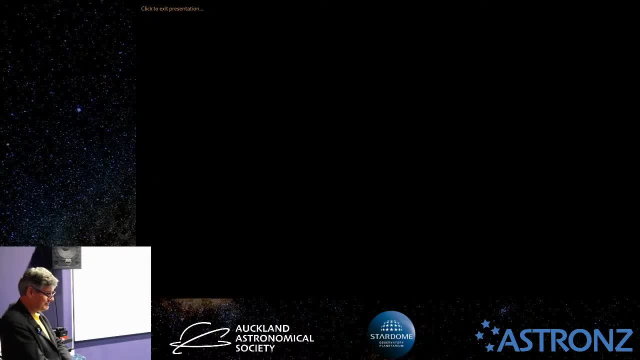 They have a look at their topics and see if there's anything that you're really interested in. We were actually just talking a bit about it just before this. Oh right, what were we discussing? It was like Tony was building a DIY autofocuser. 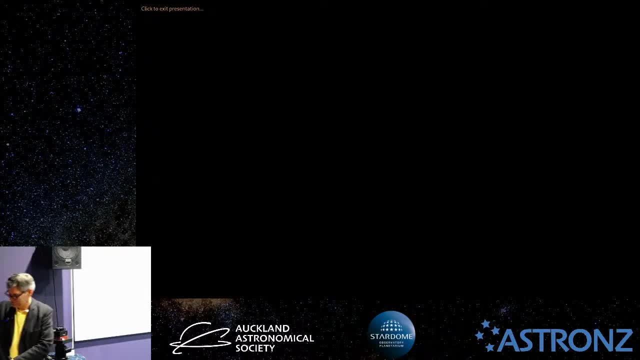 so you get to see all the interesting things. No, we missed that. yeah, I missed it. Some of the people were here, So, yeah, I don't know If you weren't there. basically, what he'd done is: 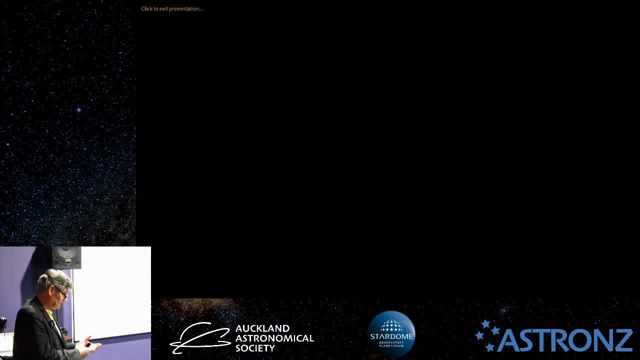 he's got a normal DSLR lens and you probably, if you're familiar with them. they have a focusing ring on them for manual focusing. If you turn autofocus off then you can adjust the focus yourself, But he wanted to be able to do it from his laptop. 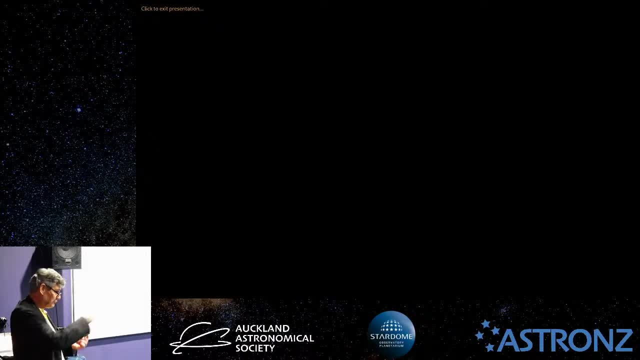 so he's built a belt that goes around that, the focusing ring on the lens, and a little motor and a connection to his computer so he can control the focusing of the lens from the computer. So quite an interesting project. So we do have one comment, another question. 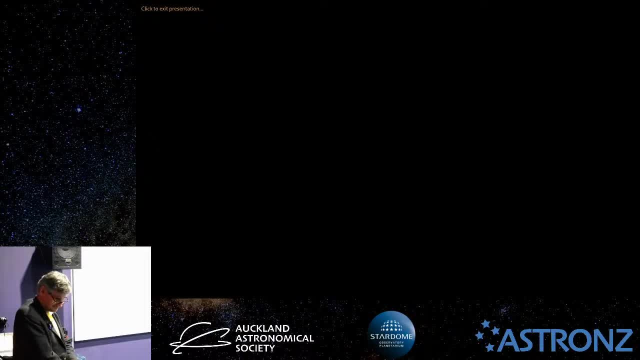 on the chat from John Drummond. He notes that PixInsight has a very steep learning curve. There are many excellent video tutorials and a book by Warren Keller called PixInsight can help the learning process, but it's a very powerful programme. 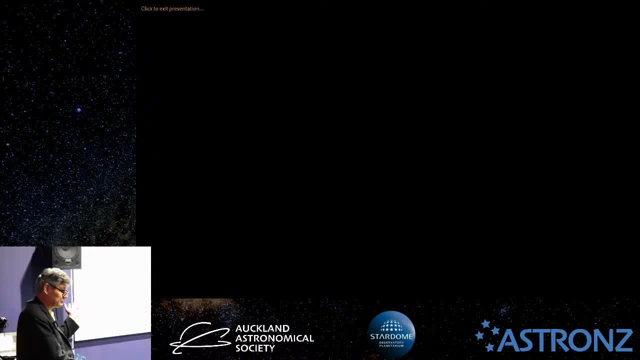 Yeah, if you're interested in even those freeware programmes, if you have a look on YouTube, there are a lot of people who have done videos on how to use these programmes and what settings to use and for different kinds of situations. So if you're getting into it yourself, 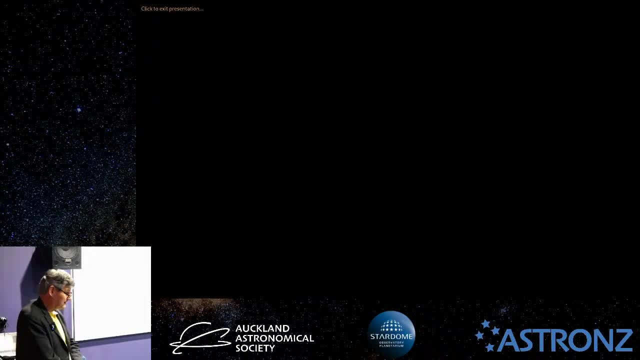 then, yeah, there are really great tutorials available that people have taken the time to do. Can't vouch for any of them, but I'm sure some of them give really good tutorials. Oh sorry, Is there a question there? Yeah, 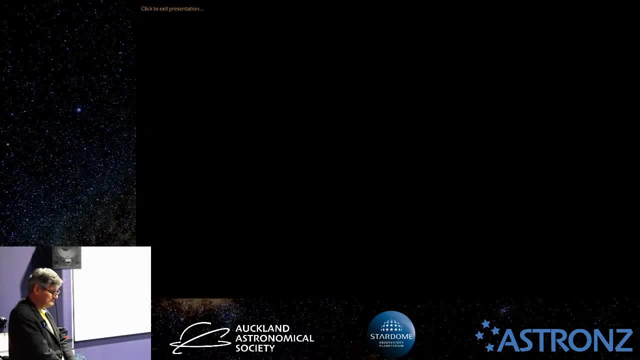 I just had one here, The last slide you had about the, about the darks and the flats and so on. so I've never worried about flats previously, but you were saying about taking a photo of the zenith after sunset. Isn't that going to have sort of a darker one side to the other? 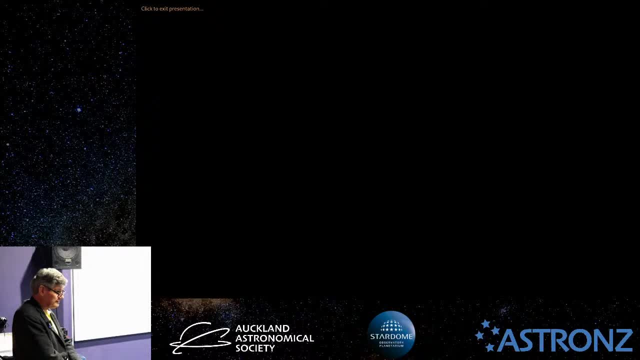 It would do. Yeah, there will be a gradient. What do you On a telescope? you probably don't have much gradient because you're looking at a fairly small patch of sky. People have worked out that the optimum for taking flats is to 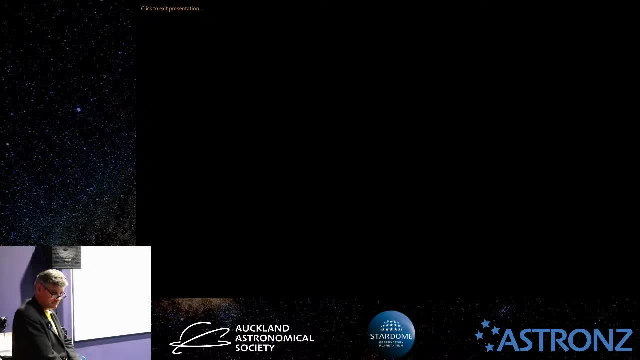 point about 70 degrees up on the opposite side to where the sun's set. So you So basically at that point in the sky you get the most uniform background. If you've got a huge field of view, like you've got a sort of short focal length DLSR or something, 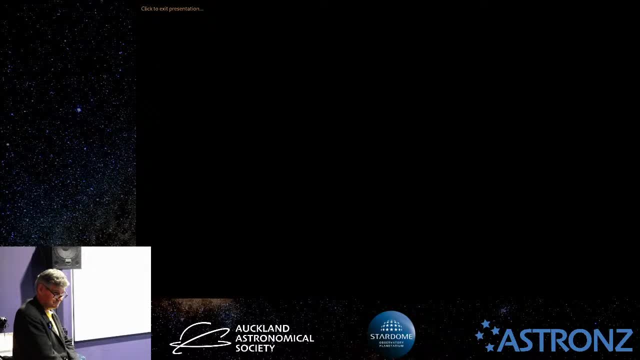 then there will be some big, quite a big variation across that field of view, Our field of view. there is only like 15 or 20-odd minutes, so it's flat as on that scale. but professional surgeries that often have big CCDs. 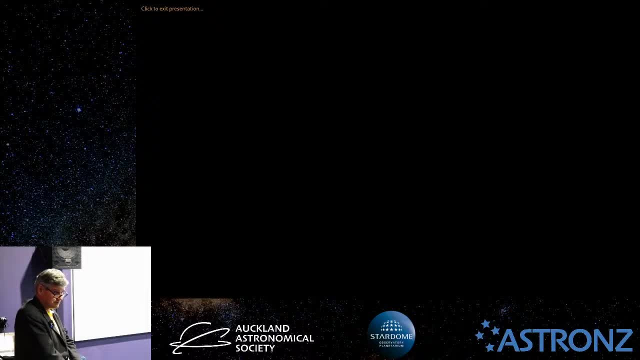 that's a rule they basically follow, isn't it? Yeah, so for a wide-angle lens, they may not be that worthwhile because of the gradient and the brightness You can- This is going a bit crazy, but you can buy electro-fluorescent screens. 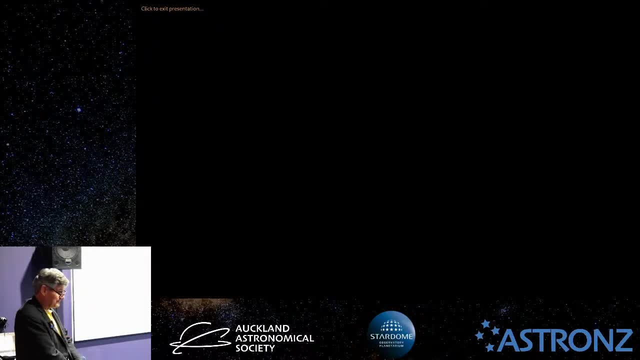 which are really have a really even illumination, and you just could take a picture of one of those. I don't know how expensive they are, Does anyone know? Not that expensive, Not very expensive. Yeah, so that is an option. 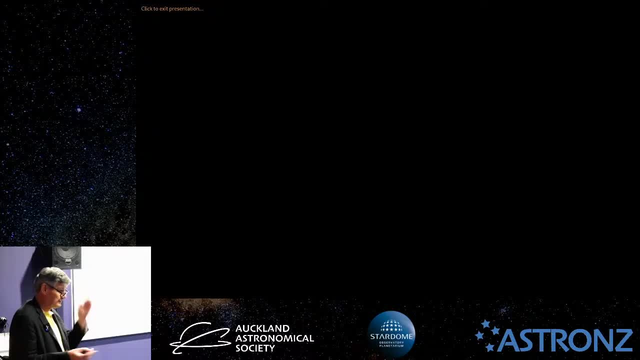 to get around the problem with sky flats with a really wide angle. The other thing is you don't just take one, because you might be unlucky and get a really bright star in the field. so you basically take a few of them, movejoggle them around a little bit. 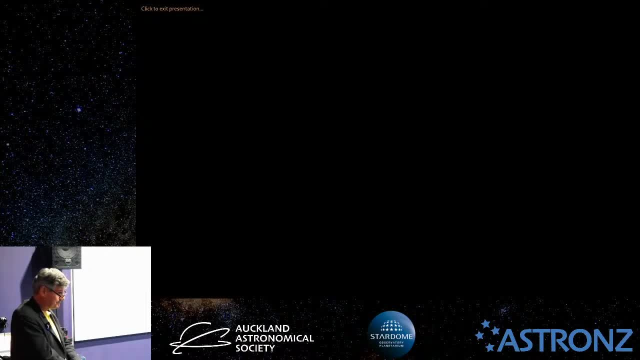 and then you Could you just put a bit of grey on your laptop or an iPad or something and put it on top. Yeah, that would probably work. yeah, If the screen is a good quality screen with even illumination, you could use that. 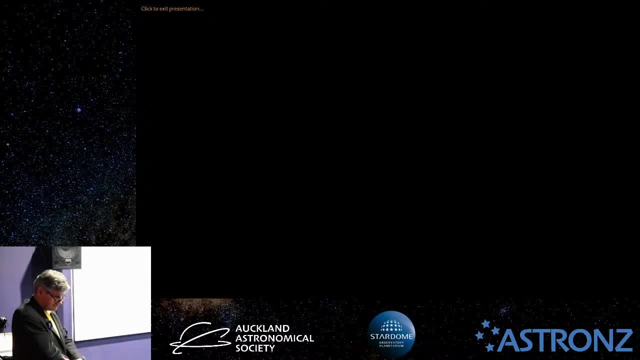 You need it to be the size of your aperture though. so if you've got an 8-inch telescope, don't hold your laptop up, because you're going to have the edges cut off. Yeah, yeah, yeah, It's got to be a big enough screen. 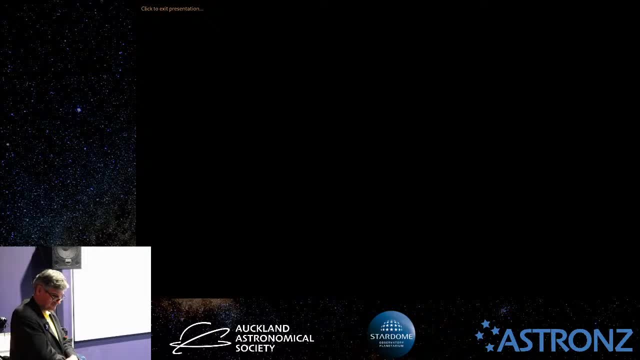 There absolutely are people who use old TVs. The backlight's pretty consistent. Some of the new ones are actually pretty nice. Some of the new really thin LED backlight ones aren't very consistent. Some of the older fluorescent-like backlight TVs are actually pretty good. 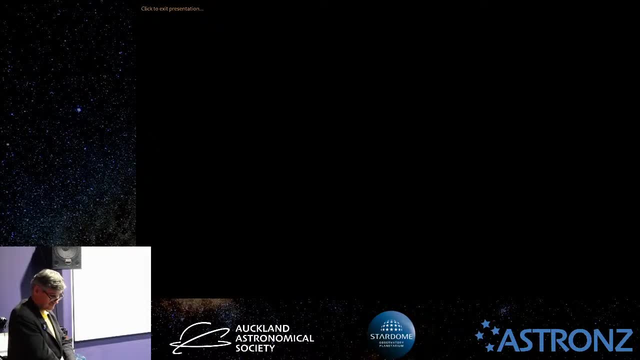 So I've seen people use broken TVs with the LCD panel thrown away, just using the diffuser panel on the back. So I've seen that done. Hmm, OK, Anything else in that case, Well, thanks for coming along, and I won't be here. 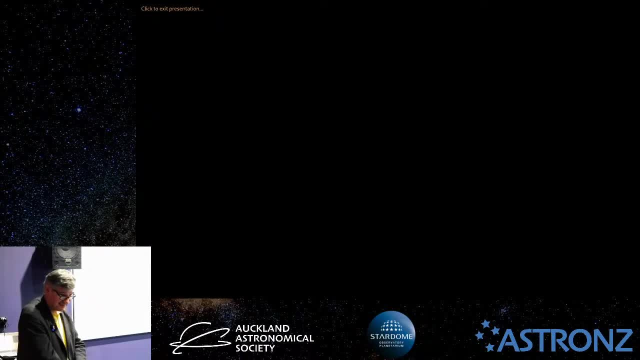 next week because I'm going to be in Wellington. but Oh no, I might be. No, I will be still in Wellington on Monday. so So poor old Gavin will have to look after things himself. Put your mask on the plane now. 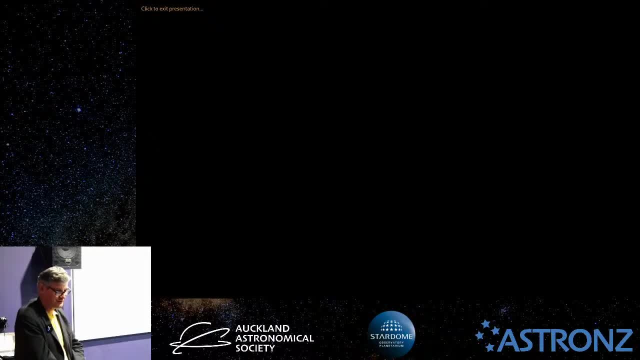 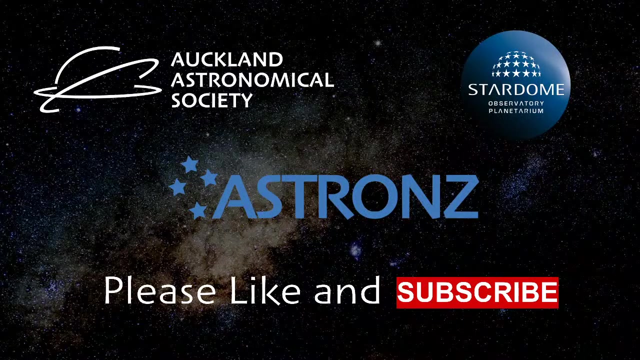 Oh, we're driving. We're going to visit Marilyn's parents as well. OK, thanks everyone. Thank you. Subtitles by the Amaraorg community.